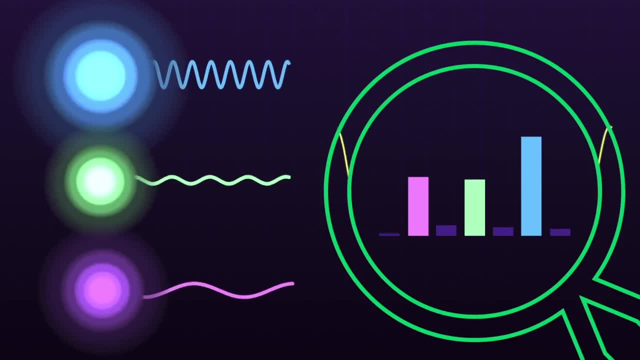 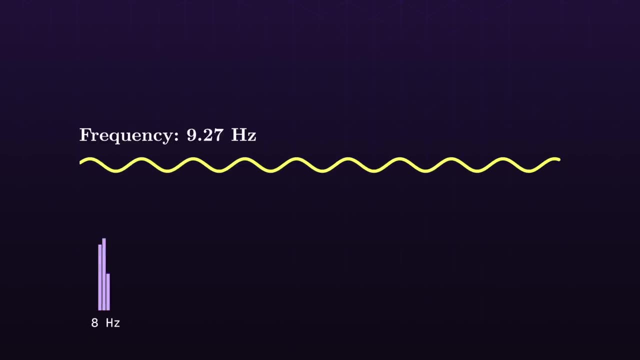 What you and I are going to talk about today is a small but essential piece of how this fundamental idea of representing a signal with its frequencies works. The core concept involves, arguably, one of the most important algorithms in modern technology: the Discrete Fourier Transform, or DFT. Most people who learn about the DFT for the first time often 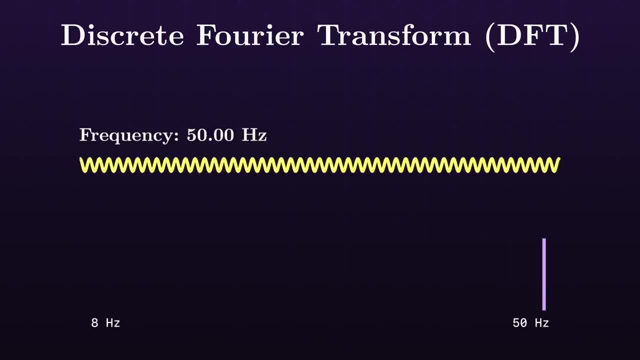 find it initially difficult to grasp. It's a complex topic that's hard to teach. The goal of today's video is to give you an idea of what the DFT is and how you can use it to improve your signal processing skills. The goal of today's video is to attempt to see if we can. 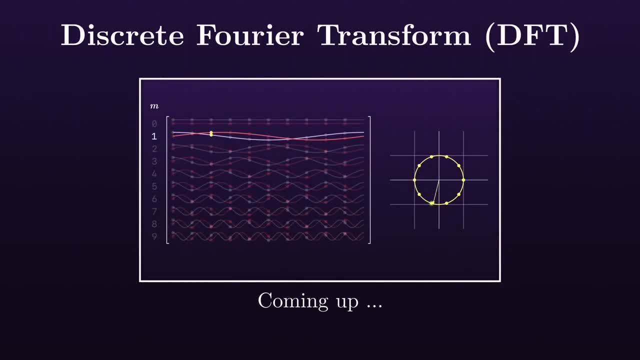 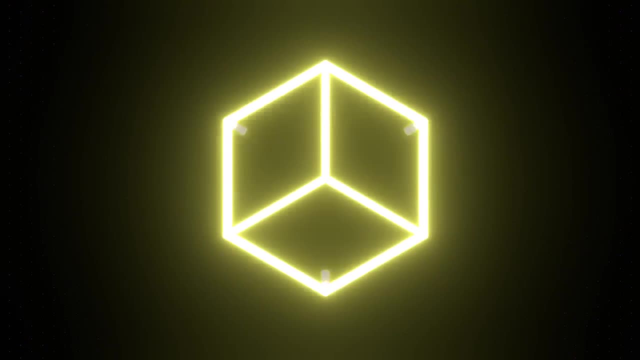 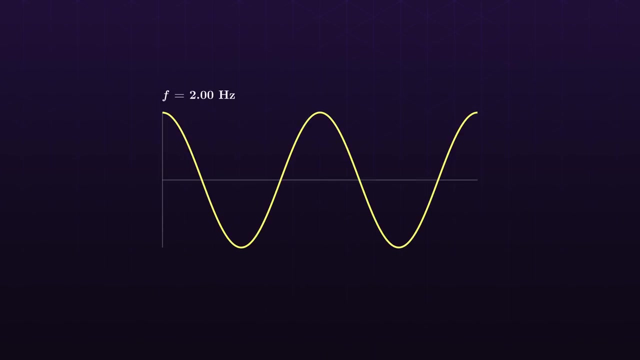 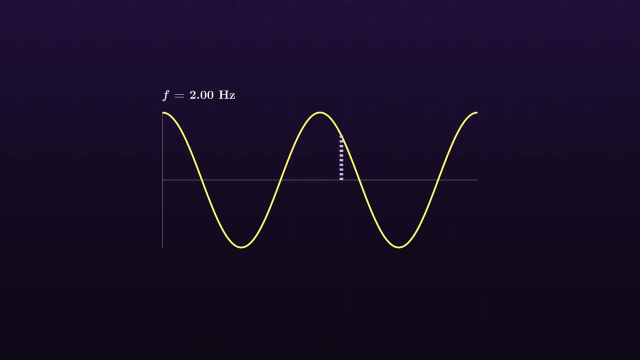 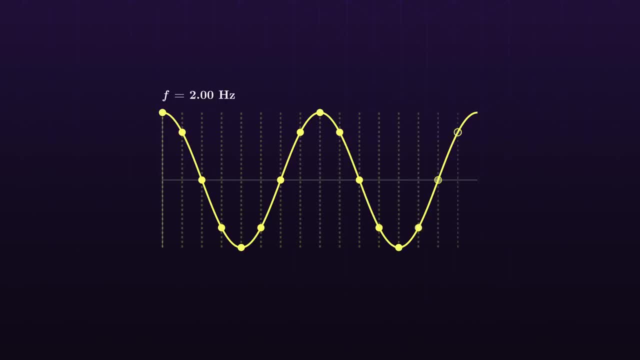 So naturally, what we have to do is sample points from the signal. The most common sampling scheme is to uniformly sample these signals to get a sequence of points that represent the original continuous signal. But there's a lot of nuance involved in sampling continuous signals. Here's a fun thought experiment. Let's say I give you a cosine wave with frequency. 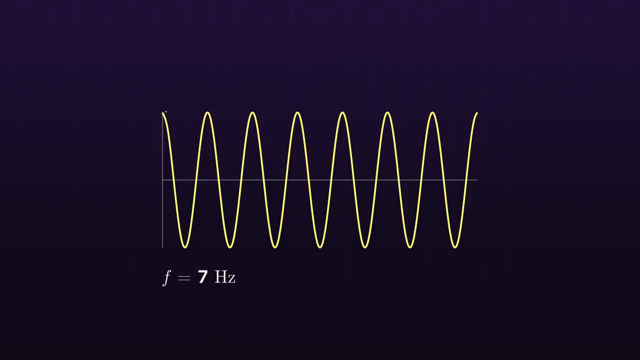 frequency: 7 cycles per second or 7 Hz. How many points do you think we need to accurately capture this signal? Think about it. it's not an easy question. by any means, Let's start by ruling out possibilities. Can we get away with representing the signal with 7 evenly sampled points? 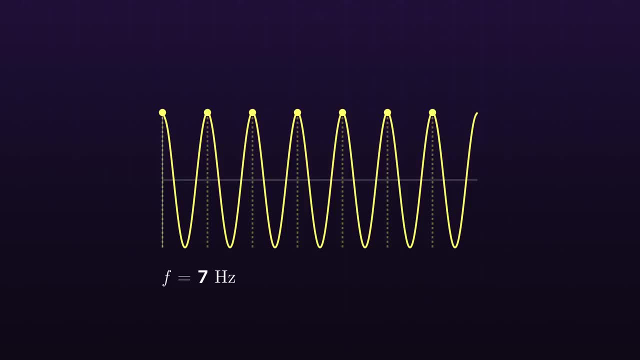 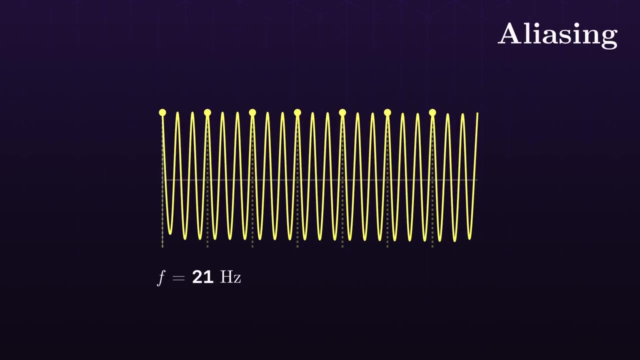 Well, one way to quickly see the issue here is: if our sampling scheme happens to, unfortunately, sample every peak of this wave, the subsequent signal looks just like a constant signal. This, by the way, is commonly called aliasing. If we sample too few points, there are many possible signals that could produce the same. 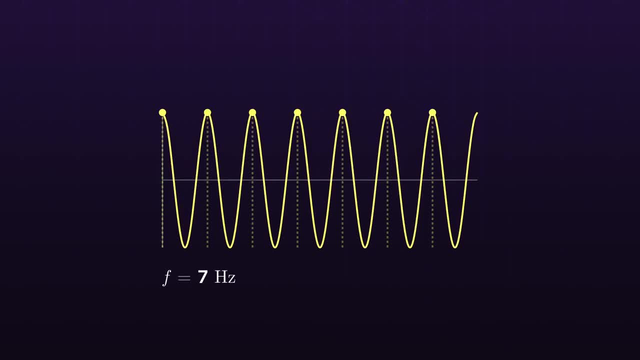 samples that we obtain. Okay, so one way to think about this is we probably need to find a way to sample both the peaks and the troughs. So is there a way we can get away with sampling 14 points instead of 7?? Funnily enough, there's a way to even break 14 points. 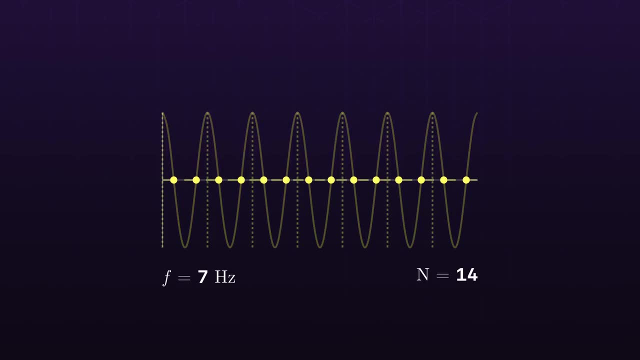 If you happen to sample evenly, such as this, once again you get a constant signal, It turns out the correct answer for this question is 15 points. If you sample 15 points in any uniform manner, you're guaranteed to accurately represent this 7 Hz signal. 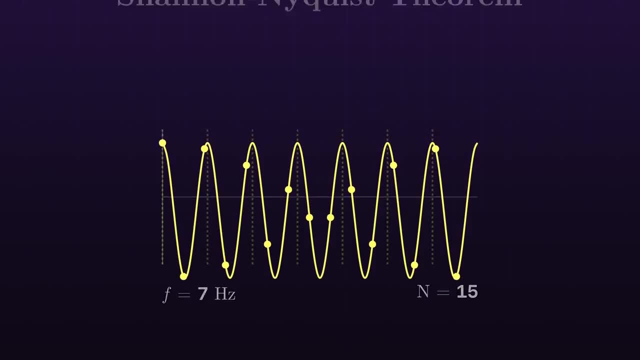 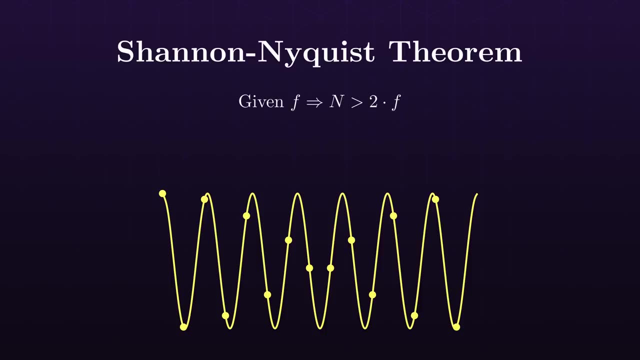 This is an example of a quite famous theorem in signal processing called the Shannon-Nyquist Sampling Theorem. There's a lot more material here that I'm purposely glossing over, but the important takeaway that I want you to remember is that for any signal of frequency f, we need to. 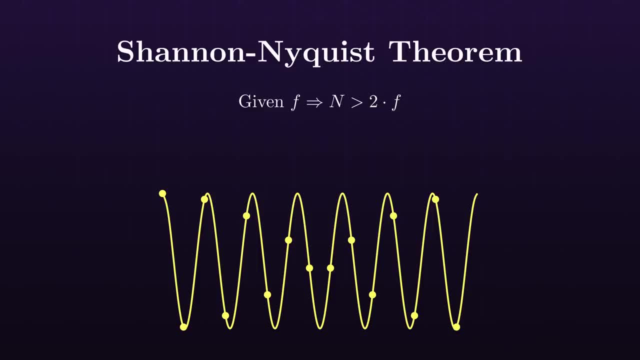 strictly have more than 2 times that frequency. 2 times that frequency, f sampled points to accurately represent the signal. Another equivalent representation is that, given n samples of a signal, the highest possible frequency that could exist within the signal is strictly less than n divided by 2.. 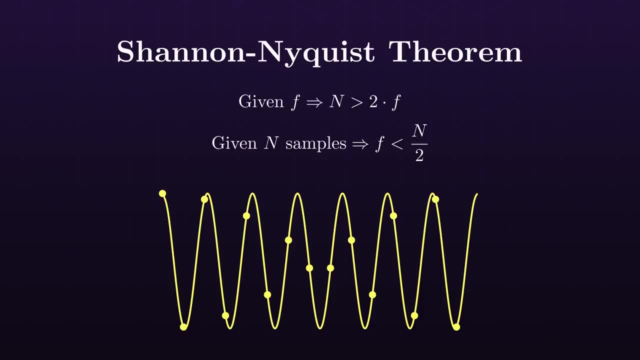 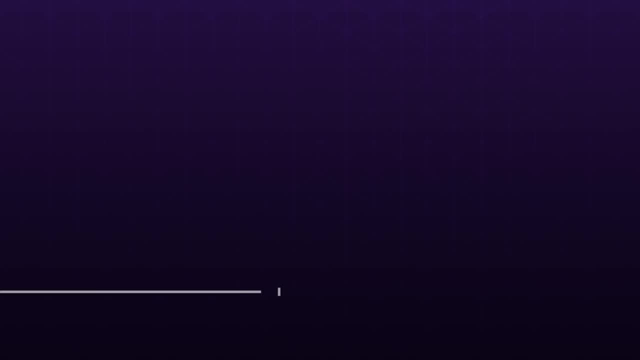 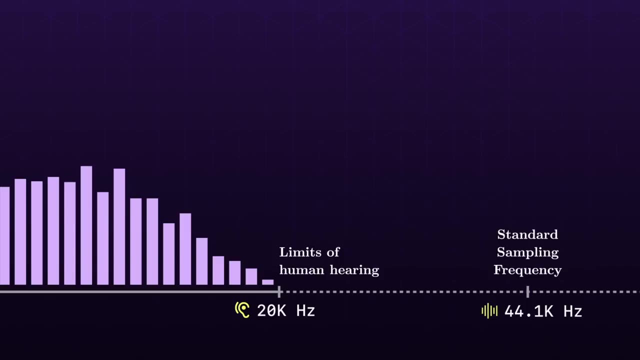 Any higher frequencies are not guaranteed to be accurately captured. This will become important later, so keep this fact in the back of your mind. One cool example of this in practice is that Most audio sources have a sample rate of at least 44.1 kHz, and the reason why is the 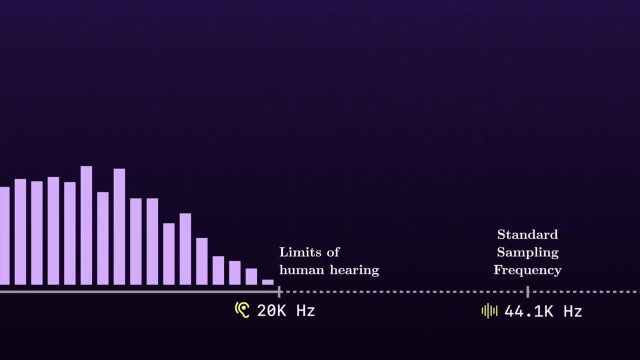 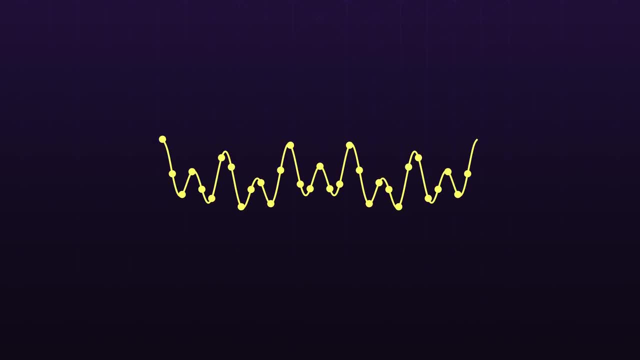 human ear generally can't catch frequencies above 20 kHz. These samples taken from the original signal give us a clear understanding of how the signal changes over time. What we showed with equalizers is another representation of the signal, but in terms of its frequencies. 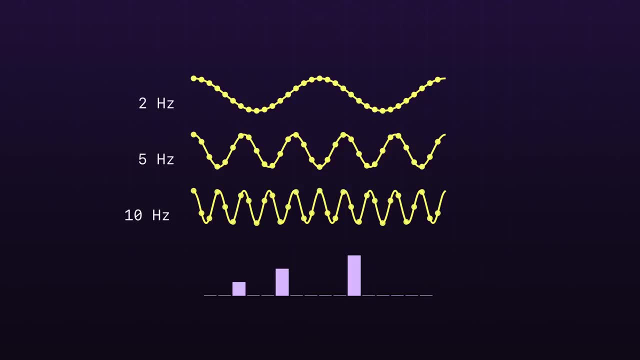 Fundamentally, these two representations give us the exact same signal. They're just two different ways of communicating the signal. The signal is a signal that is not a frequency. The signal is a frequency with slightly different frequencies, and things like that. 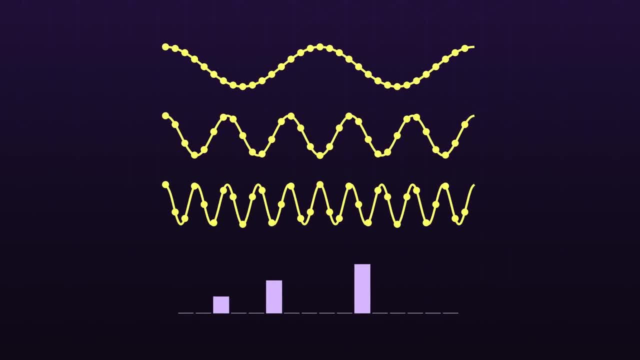 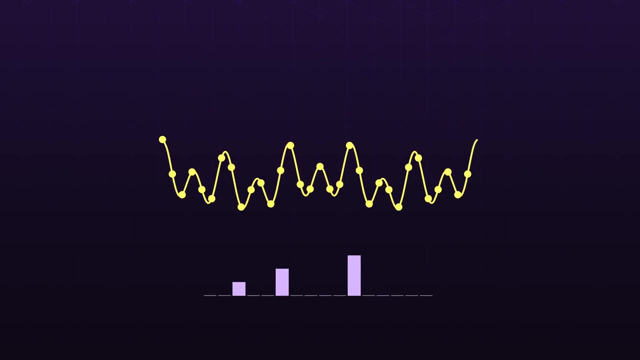 What this frequency representation tells us is that this particular signal is composed of three different waves of frequency: 2, 5, and 10Hz. The idea of this frequency representation is: if we take these three waves, scale them by their relative strength and add them together, we will get the original signal. 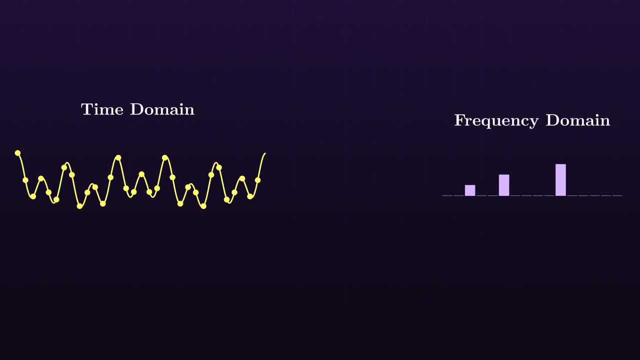 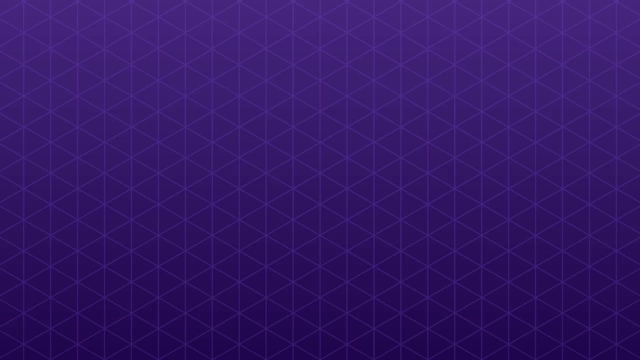 This is the core idea of what's called a frequency domain representation. Do you get it? It's extraordinarily important that we understand that frequency domain representation is an important thing. understand that all the DFT involves is a conversion between a time domain representation to a frequency domain representation. 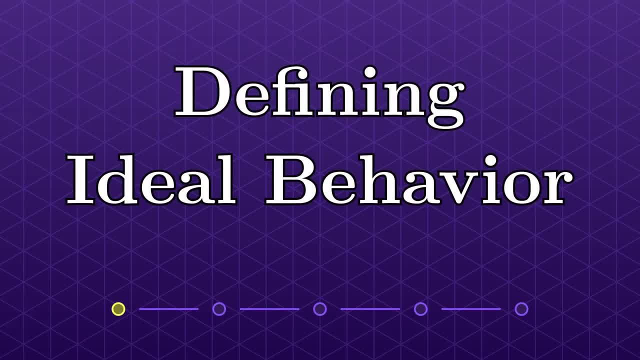 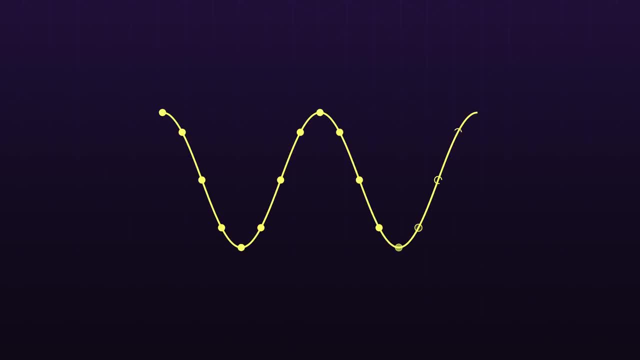 Whenever we want to understand how we might rediscover a complex idea, it really helps to have an understanding of how we would like it to behave. for some simple examples, Suppose we have a cosine wave of frequency 2 Hz. Ideally, what we would like the frequency domain representation of such a signal to be is a. 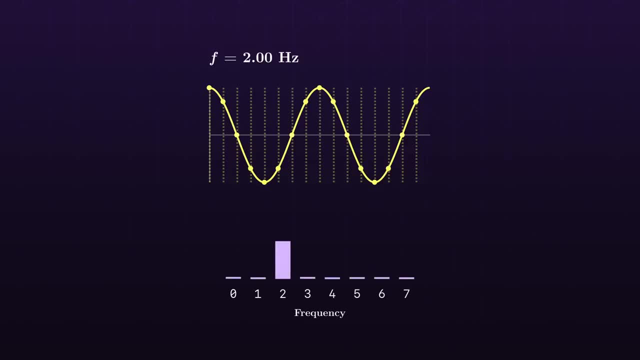 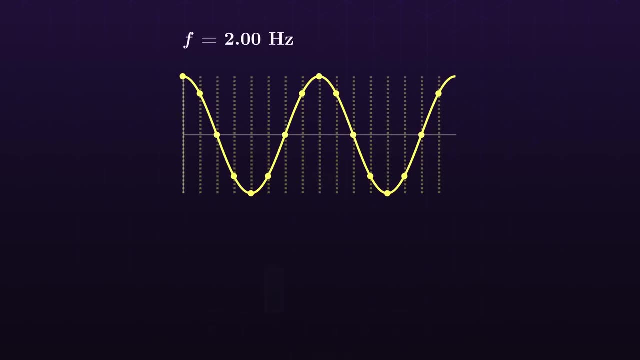 peak at the frequency 2 and zeros for all other frequencies. So, in the context of this simplified example, we're looking for some operation that produces a high value for an input frequency of 2 and zeros for all other frequencies. What that means is the operation we're looking for is fundamentally a measure of similarity. 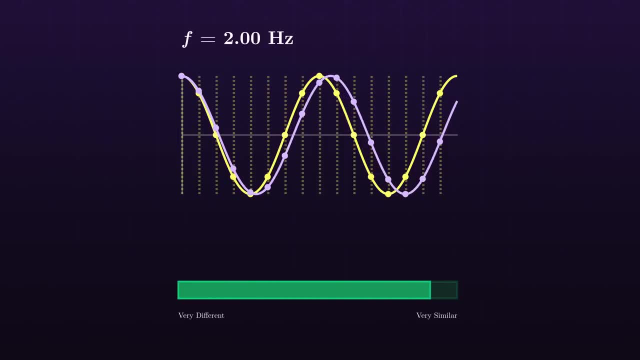 When the frequencies match we should get a high similarity score. but when they have different frequencies we ideally want a score of similarity, So we can get a high similarity score. Given a sequence of input points from a time signal, we can essentially represent the sequence. 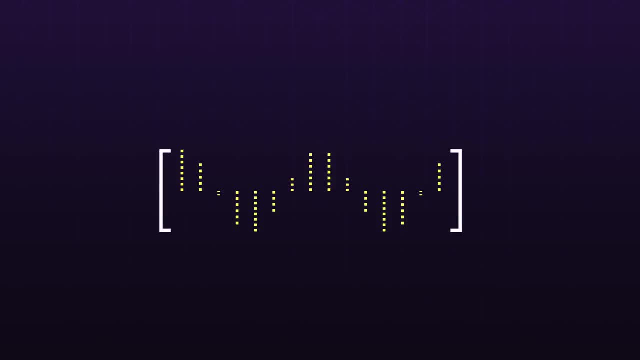 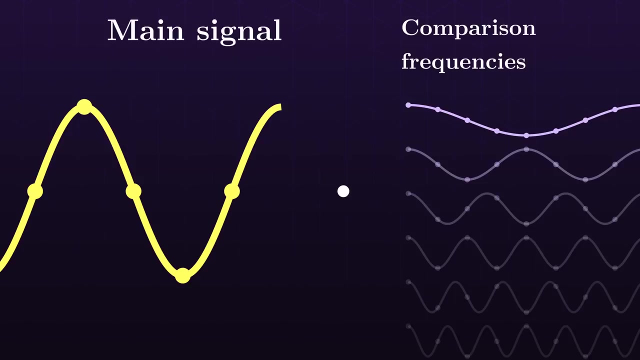 as a vector. Now, one of the most common ways to represent similarity within the context of vectors is the notion of a dot product. So let's start our analysis by seeing how we can properly construct a similarity measure for our original time domain signal and different frequency cosine waves. 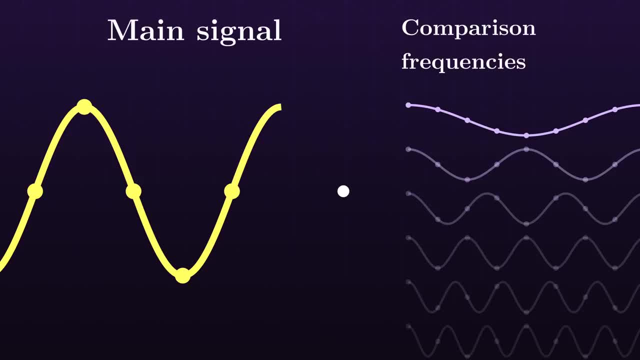 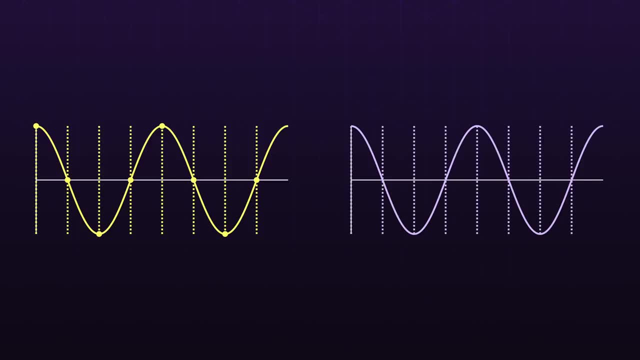 In order to properly construct a dot product, we have to first get a value of time. For a dot product. we need a set of samples from the cosine waves that we want to compare with. As a first attempt, it seems reasonable to sample the cosine wave at the same sampling. 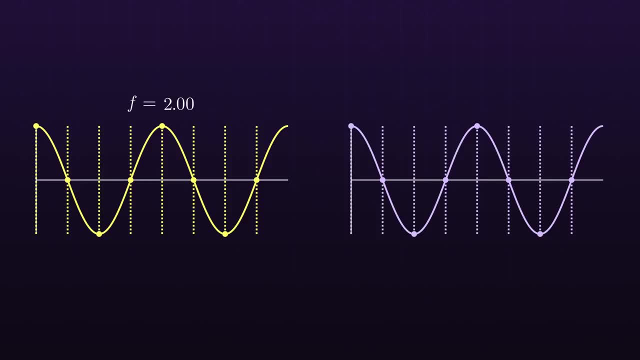 rate as the original signal. And this does work well when the original signal and cosine wave match one to one, as it does here in this simplified example. But what about other frequency cosine waves? There are theoretically infinitely many cosine waves that we could compare to in this time. 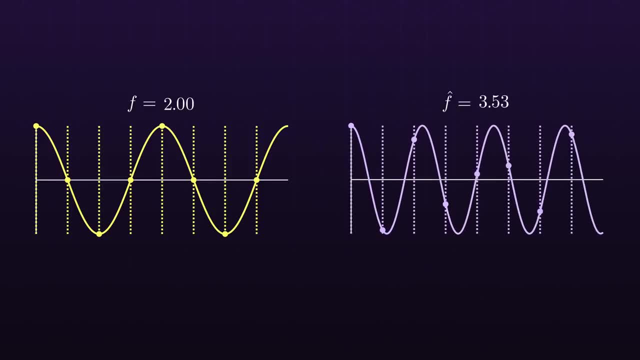 segment and we can't evaluate all of them. So how do we go about doing that? Well, first, let's start by picking a set of frequencies to compare with. To be clear, there are inherently two frequencies involved. One is the frequency of the original cosine wave and the other is what we'll formally 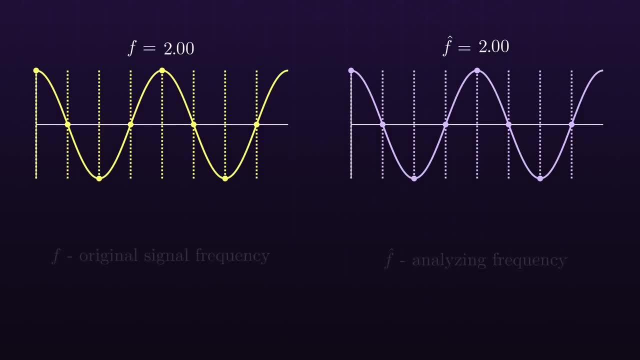 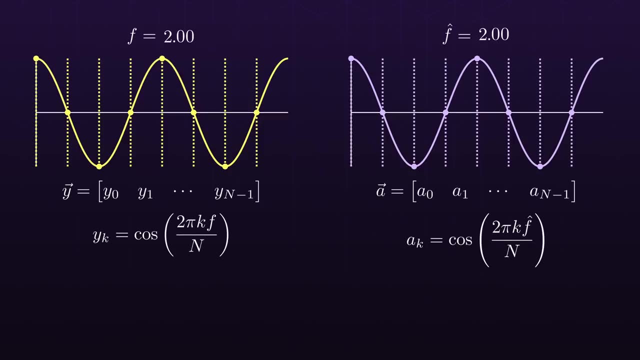 call an analysis frequency For any analysis frequency f hat. we'll currently define it as a cosine wave with amplitude 1 and frequency f hat. So when picking frequencies we want to compare against. remember a key property we're looking for in our frequency domain: representation. 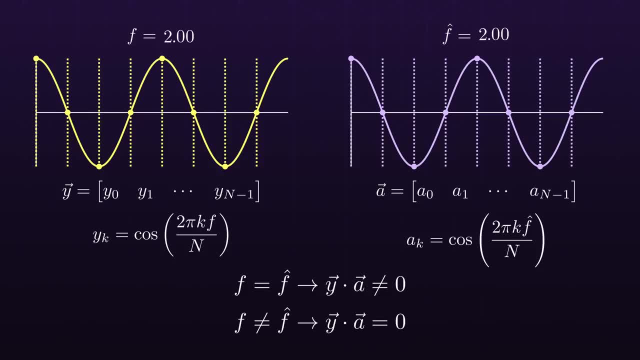 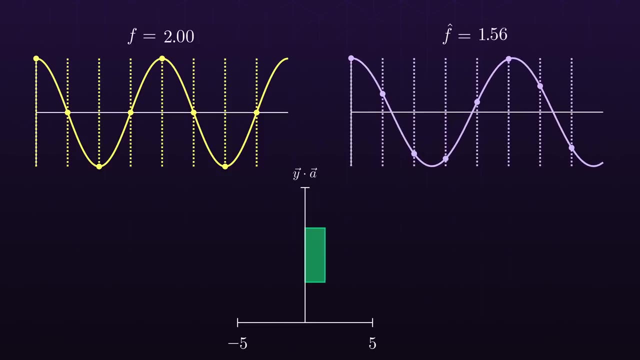 We want all frequencies other than the intrinsic frequency to have zero contribution. So let's see what happens when we take the dot product of this cosine wave with other frequency cosine waves. Here we'll slowly adjust the analysis frequency and observe what happens to our similarity. 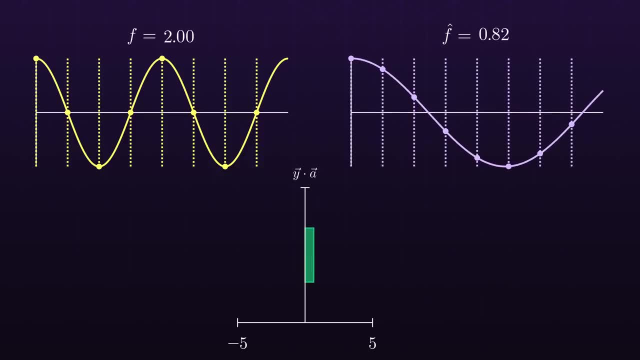 measure. One thing to notice here is that if you take any random cosine wave of some real number frequency, the contribution is actually almost always nonzero. If you take any cosine wave of some real number frequency, the contribution is actually almost always nonzero. So we can see that if we take any cosine wave of some real number frequency, the contribution 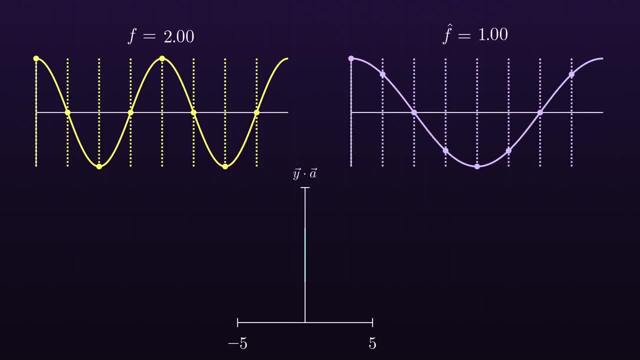 is actually almost always nonzero, But there are a specific set of frequencies where things just perfectly cancel out and we end up with the contribution of zero, as we desire. What's interesting from this particular example is that when our analysis frequency is defined such that there is an integer number of cycles within the time range provided, 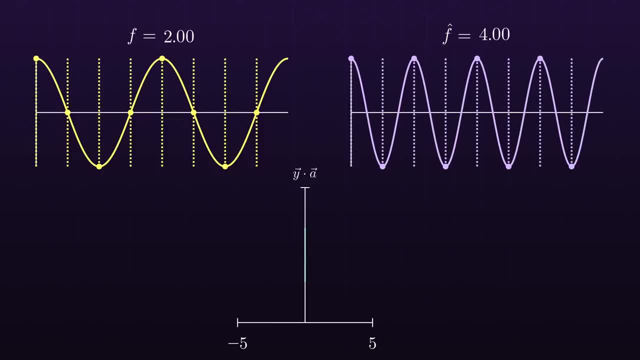 the similarity measure seems to always end up being zero. This looks kind of promising, so let's dive a little deeper into this behavior. So far, we've been able to see that the frequency of the sine wave is always nonzero, and the frequency of the sine wave is always nonzero. 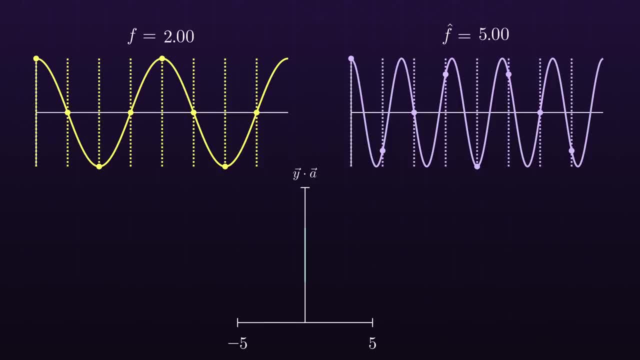 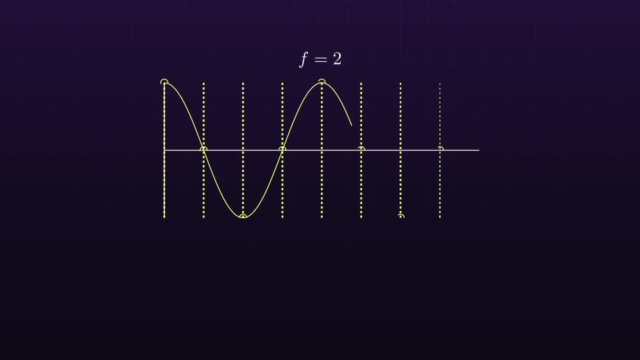 So far, we've been quite hand-wavy with our treatment of what we're looking for in the DFT. To go one level further, let's formalize things a little bit more carefully. Right now we have a time domain signal which, as mentioned, can be represented as a vector. 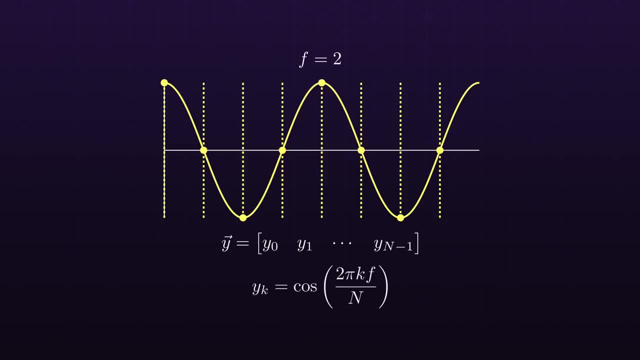 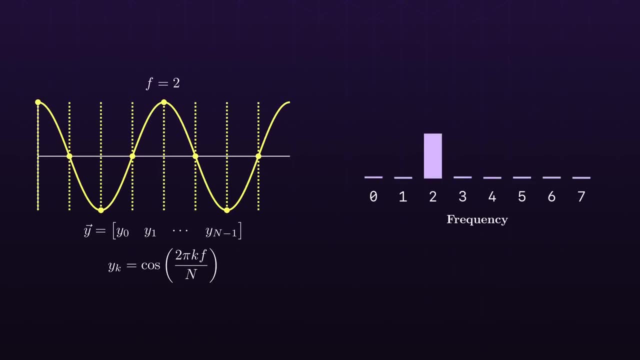 of sampled points. We want to define some transformation that takes this time domain signal and gives us a frequency-based representation where a certain set of frequencies is mapped to a value that represents a contribution of that frequency to the original signal. We already asserted that for a simple cosine wave with frequency f, how we want this transform. 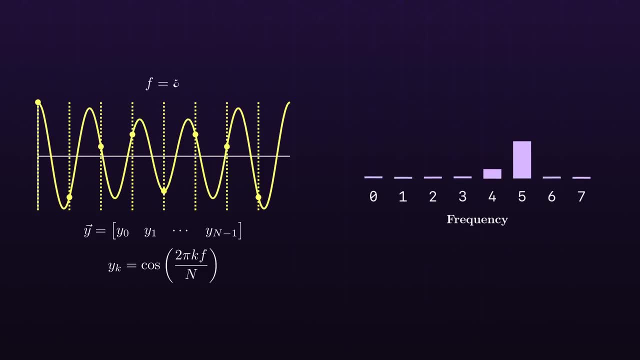 to behave ideally is to have a high value for that frequency f and zeroes for all other frequencies. We saw some promising signs of this behavior as we compared our cosine wave to different analysis frequencies. Currently we have a similarity measure that's defined as a dot product between our original. 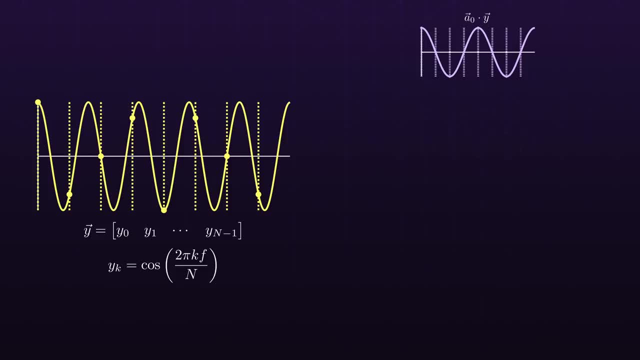 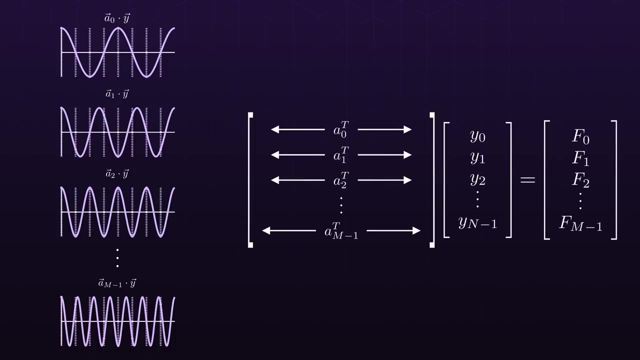 signal and sampled points from an analysis frequency, and what we're looking for is performing this operation across a set of analysis frequencies. So let's take a look. What sort of transformation operation expresses this really well? What we're essentially trying to define is a matrix vector product. 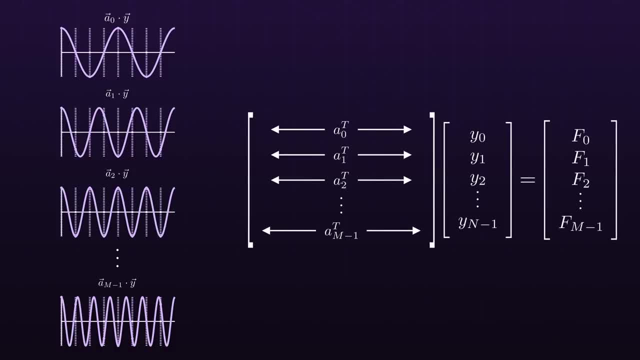 By representing samples from different analysis frequency cosine waves as rows of this matrix, we get a compact representation of our dot product similarity measure applied to all analysis frequencies. What we're ideally looking for is three fundamental requirements to be satisfied in this specific example of a single frequency cosine wave. 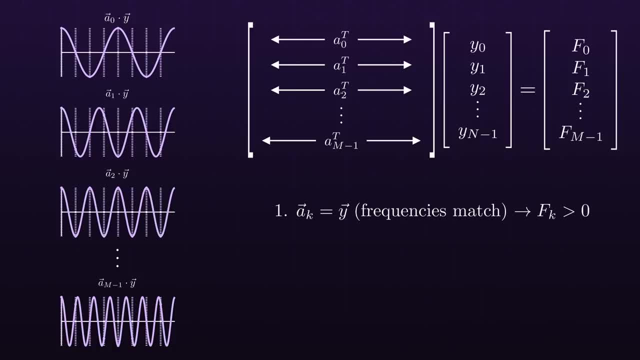 First, we want it to be the case that when the analysis frequency is exactly the same as our original signal's frequency, the respective frequency domain values should be greater than zero. And two, when we compare against analysis frequencies that have some other value than. 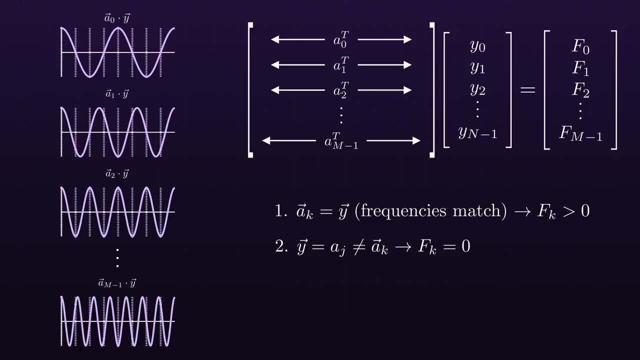 the original signal's frequency, we should get a corresponding dot product of zero to signify that there was no contribution of those frequencies to the signal. And lastly, we would like to see that our original signal's frequency is exactly the same as our original signal's frequency. 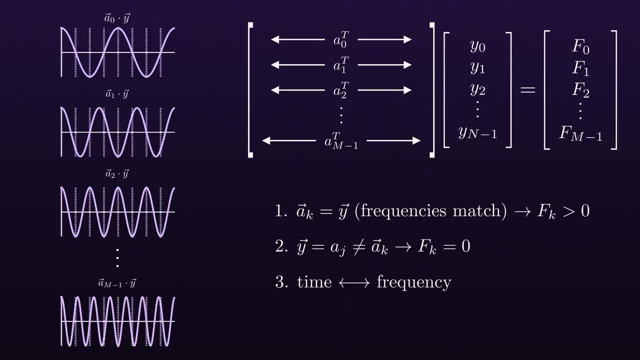 So we'd like this transformation to be reversible. Given a frequency representation of the signal, we'd like to exactly reconstruct the original time domain signal. Now it turns out these requirements can be translated to fundamental mathematical properties of matrices, Starting from the bottom. to make this operation reversible, this mysterious matrix must be. 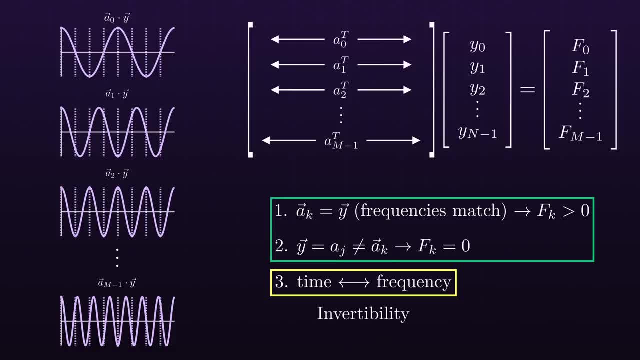 invertible. And to fit these two constraints, what we're looking for is an orthogonal matrix, So immediately off the bat, we're going to need a matrix vector, And to do that, we know that our eventual definition of the Fourier transform needs. 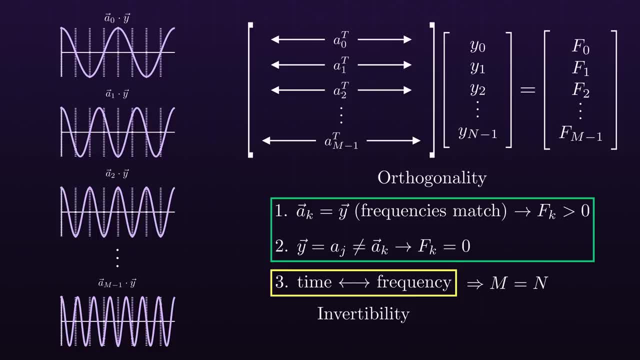 to have the same number of analysis frequencies as the number of samples in the signal. Otherwise there's no way the matrix can be invertible. Well, let's see if our earlier definition of analysis frequencies for cosine waves fits the criteria we're looking for. 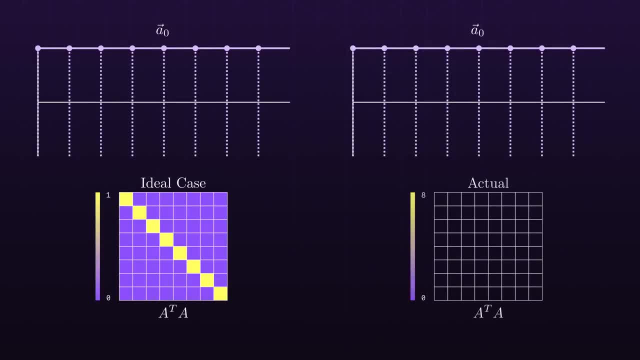 As we have seen earlier, the nice property of these sampled points from analysis frequencies of cosine waves is that when the cosine waves have the same integer frequency, the dot product is non-zero, And when they have differing integer frequencies, they have a dot product of exactly zero. 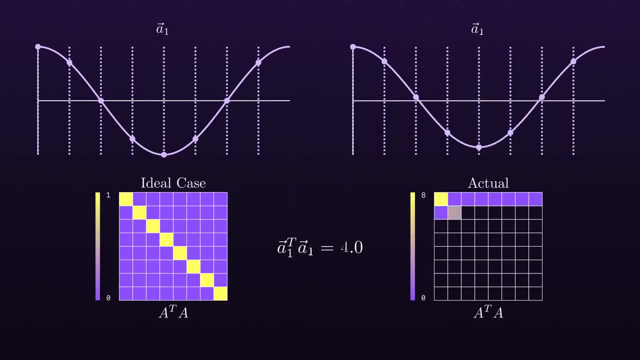 Or at least that's what I implied earlier. Some of you may have noticed that this is actually not accurate. It turns out that there are particular pairs of analysis frequencies that have a non-zero dot product, even when the underlying frequencies are different. 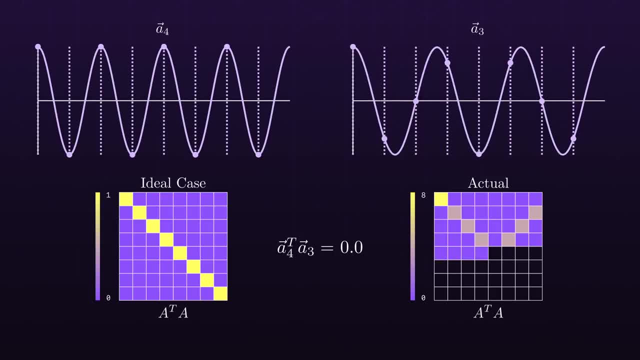 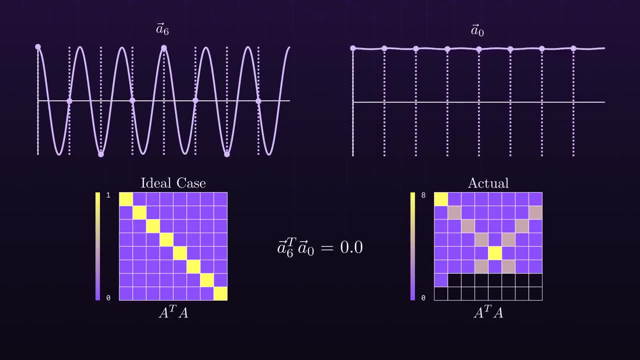 In fact, if we compute every combination of dot products between these analysis frequencies, we see an interesting pattern. For example, if we compute every combination of dot products between these analysis frequencies, every non-zero analysis frequency, there exists exactly one other frequency that results. 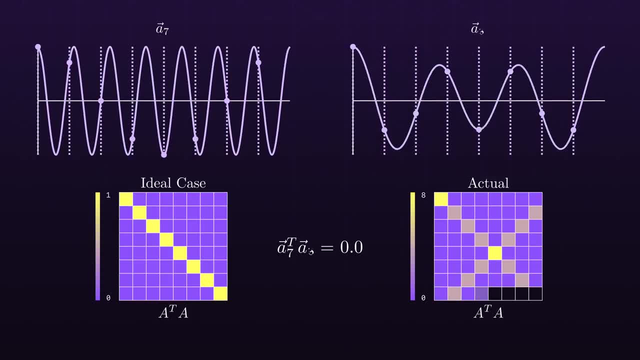 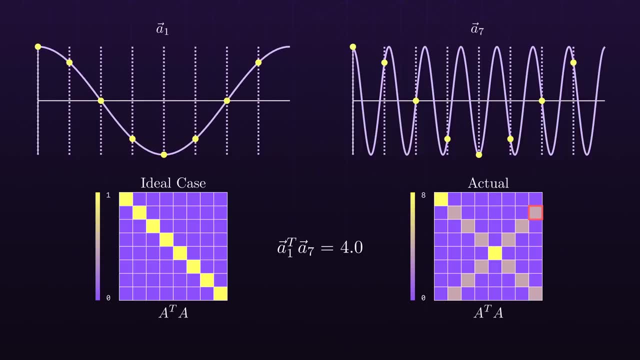 in a positive dot product. What's going on here? Well, if we pull it apart, we see. the problem is that, even though these particular frequencies have different underlying cosine waves, the samples themselves are actually identical. This is essentially a byproduct of the Shannon-Nyquist sampling theorem. 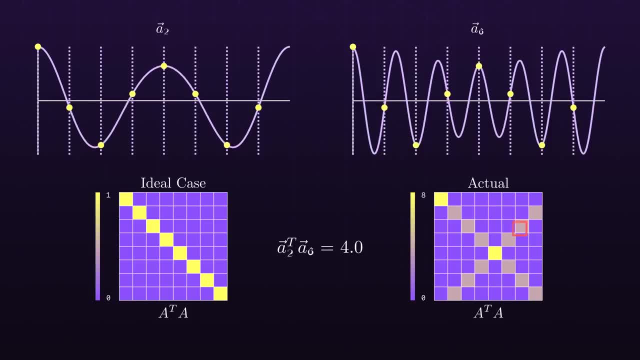 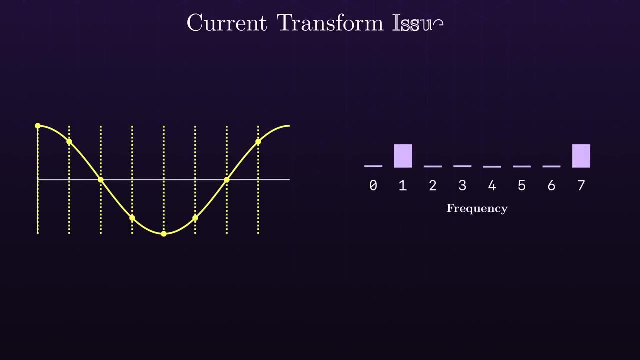 Since we're only sampling 8 points, Any frequency 4 or above cannot be accurately represented with 8 samples, so we end up with overlap. One thing that you might notice here is that a subset of this matrix is nicely defined, And one way that we can sort of get past this sampling problem is to only consider the first. 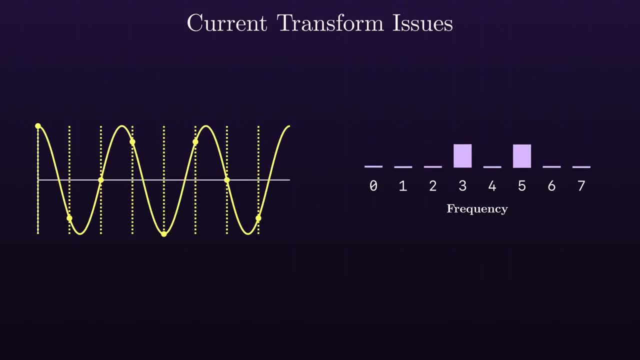 half of any frequency spectrum. When we use this transform on any non-zero frequency cosine wave, there will always be some redundant information as a result of the nature of our current definition of the non-zero frequency cosine wave. In other words, the matrix itself is not orthogonal, it's not invertible. 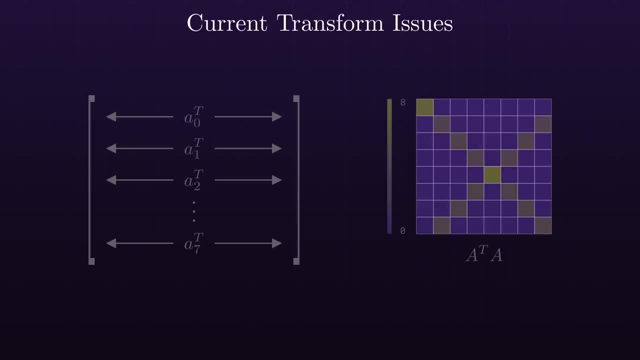 The bigger problem here is because multiple rows of our analysis frequency matrix are identical. That actually means our matrix is not only non-orthogonal, it's also non-invertible. This is, unfortunately, a serious problem. Invertibility is an essential requirement so that we can actually reverse our transform. 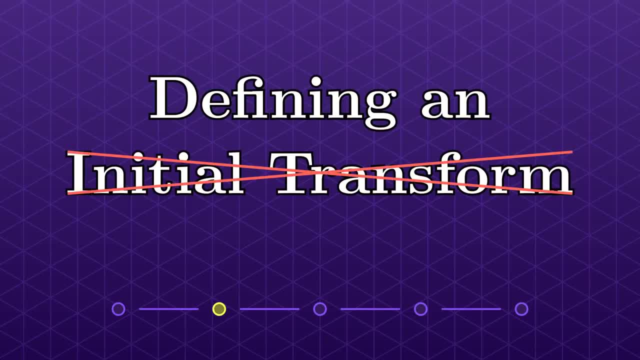 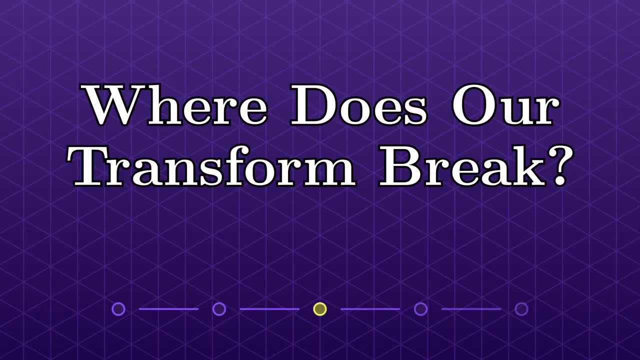 As a result- minor spoiler here- this is not the actual Fourier transform, But sometimes, from an engineering perspective, It's fun to have. it's fun to try something that we know is wrong and see where things break down Before we dive into how frequency decomposition via the DFT really works. 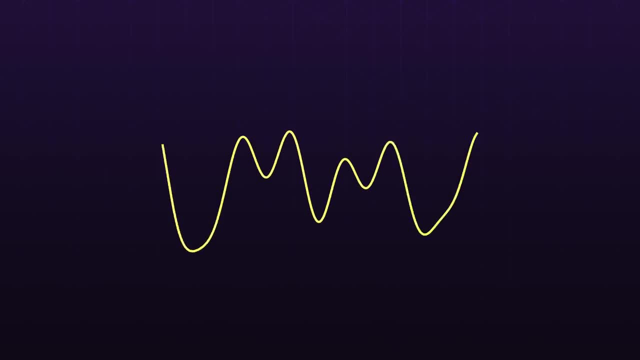 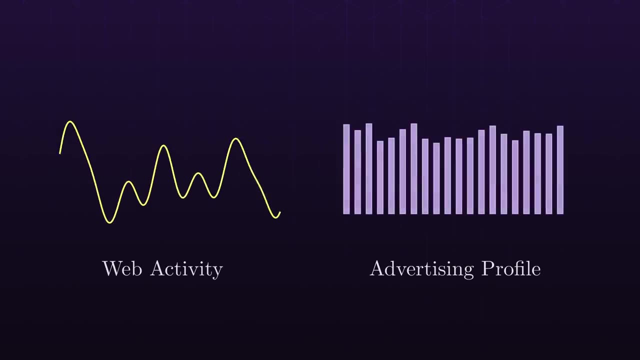 I want to take a quick aside to talk about some similar types of activity that happen on a day-to-day basis. In some countries, it is legal to monitor your internet traffic and build up an online profile of you basically taking in a signal- that's a function of web activity- and decomposing it into a fairly accurate advertising profile. 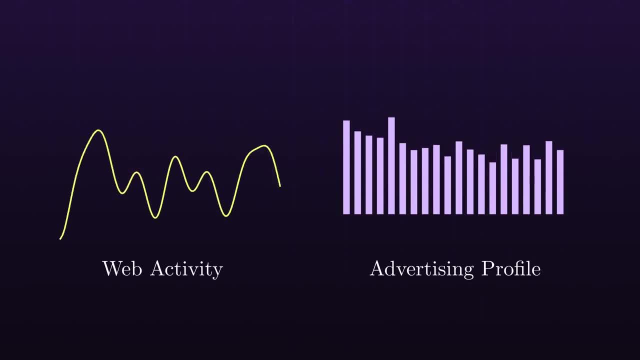 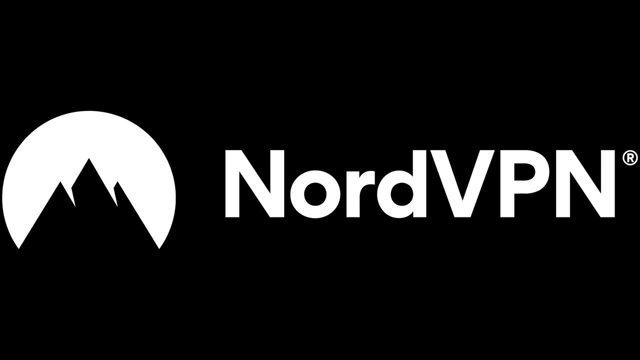 one that can perhaps also be sold and used maliciously When browsing online. this is not something any of us would like to think about, so that's why I recommend NordVPN, the sponsor of today's video. NordVPN prevents outside parties from intrusive tracking and building up such a profile. 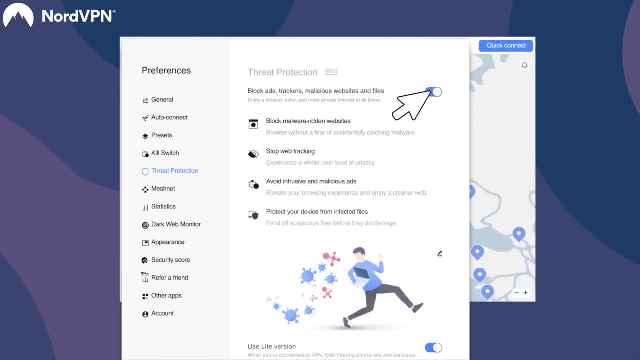 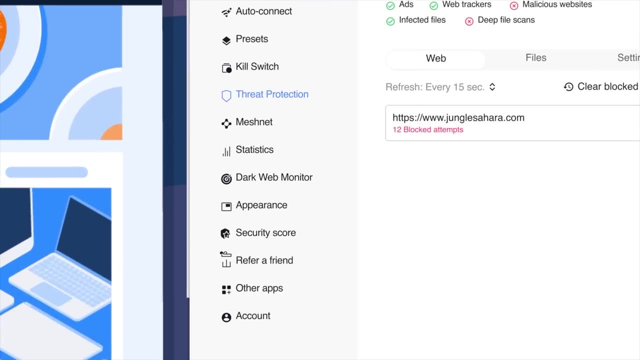 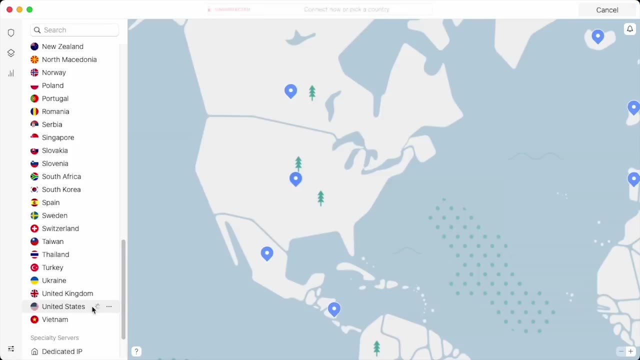 It's also great in areas where internet service providers can purposely slow down your connection. In addition to these essential features, one of my favorite uses of NordVPN is while traveling. NordVPN can give you a spoofed location in any of 60 countries, allowing you to get access to shows and entertainment that you may not usually get. 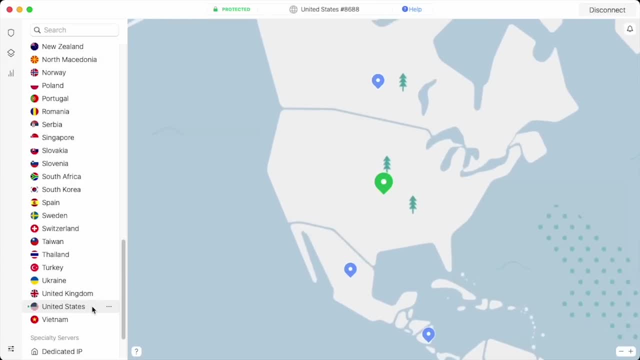 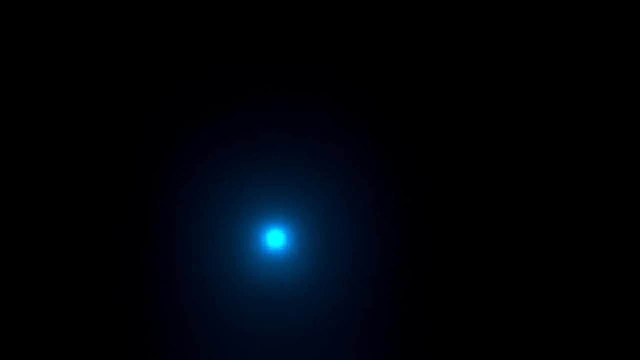 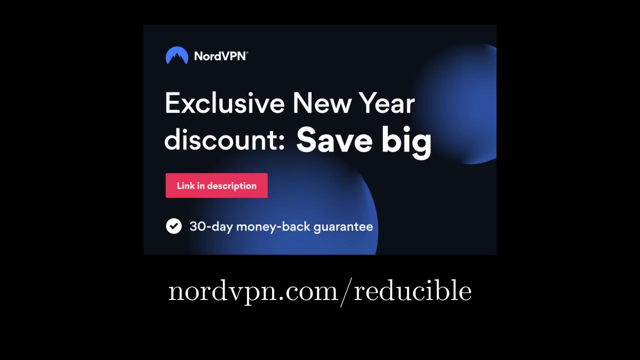 The ability to connect six devices simultaneously allows you to take these features anywhere you go. NordVPN has been in this business for years, making it easier than ever to get set up. They've built a reputation that values trust and cybersecurity. If you're interested, go to nordvpncom. slash reducible to get the two-year plan with an exclusive deal plus one bonus month free. 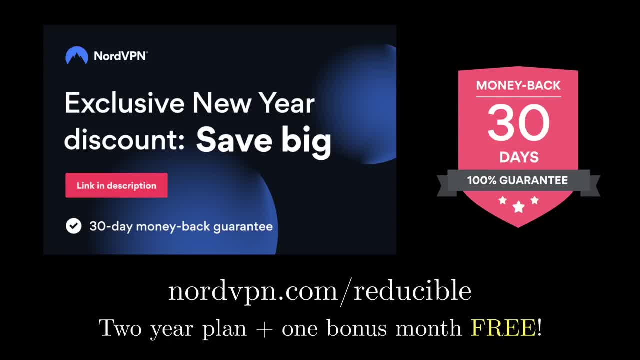 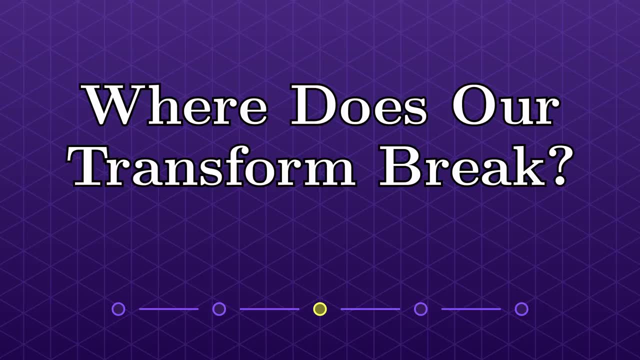 It's risk-free with NordVPN and NordVPN's 30-day money-back guarantee. Thanks to NordVPN for sponsoring this video. Going back to our previous question, we know our original transform has an issue with invertibility, and to see where things break down. 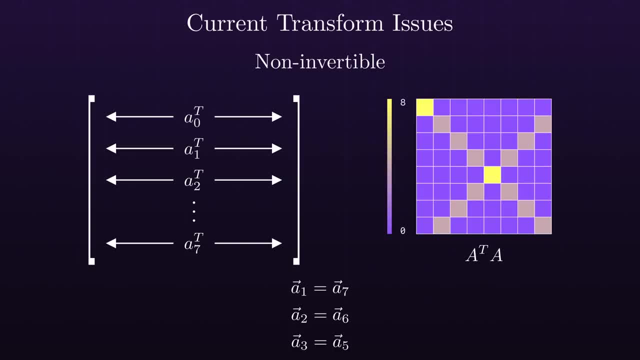 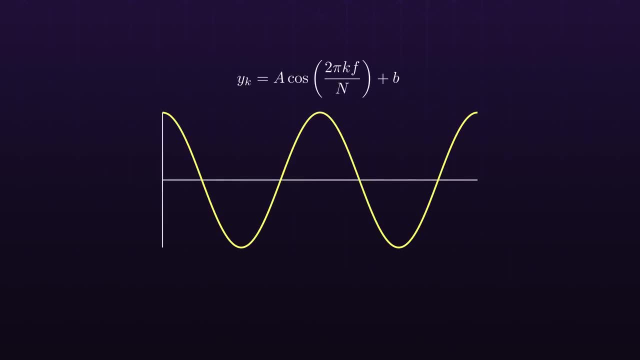 let's observe what happens when we try to apply this fake Fourier transform to a variety of signals of different definitions. Let's think about some test cases To set some ground rules surrounding our assumptions. all the transforms, from here on out, will be taken from 16.2% of the time. 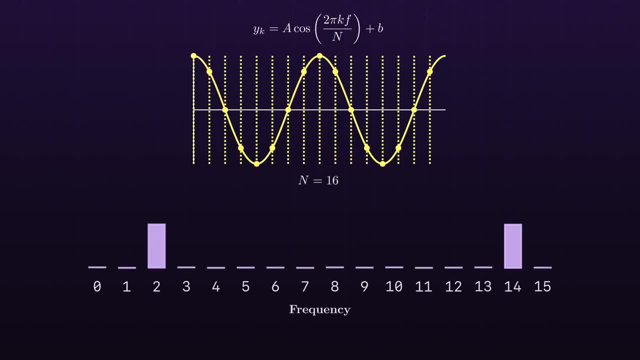 All the transforms from here on out will be taken from 16.2% of the time. All the follow-up's will take you to 16.2% of the time. No safe space and no, if you can avoid confiscating those expressions. 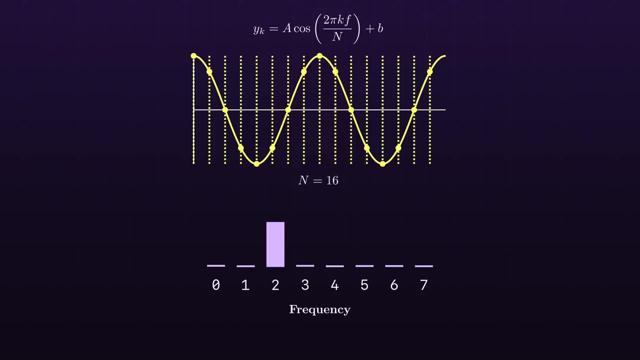 though you can still put them in the test case and freeze it as a transfer of 45% Auto Failure. E imply there's no more leftover coefficients. What we're going to do is study a partnership theory, justify value anywhere here in the esschenuse population. 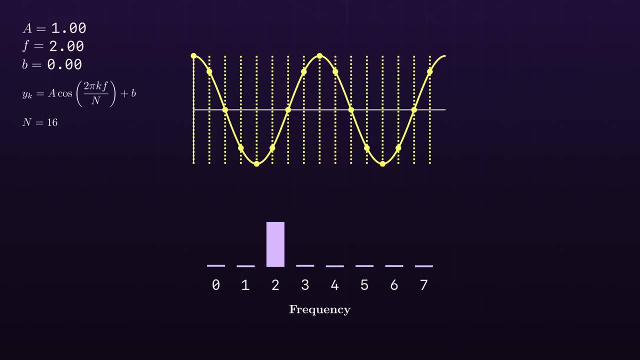 screamingactions about how this visualization works. Another study was conducted just a few months ago to assume the�� Amplitude changes do seem to be properly captured by our fake Fourier transform. The next test case is to change the frequency of the cosine wave. What we expect to happen is that 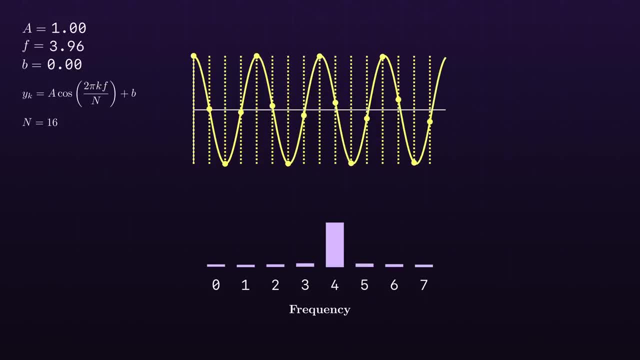 our test transform's peak will be correspondingly updated to the new frequency as our frequency changes, And indeed that is the case. The peak moves in the frequency domain as the frequency of the original signal changes. Let's see what happens when we shift the y-intercept of our 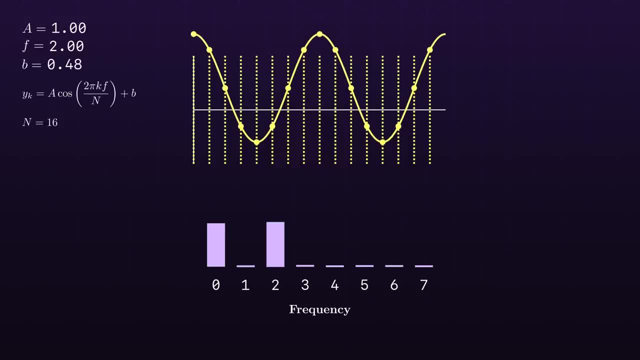 cosine waves. When we shift these waves up, we are essentially adding a signal of zero frequency, and our fake Fourier transform does encapsulate that information in the contribution to the zeroth analysis frequency. Alright, so far nothing has clearly been broken, so let's make our test. 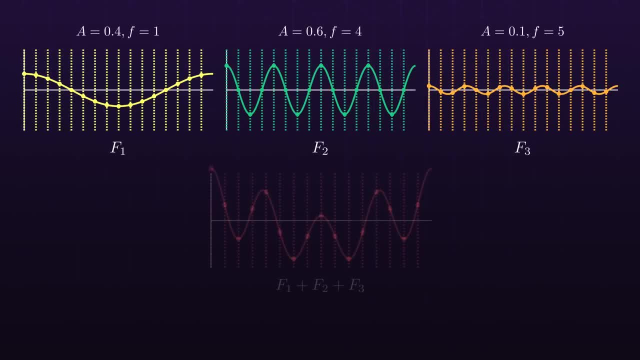 cases a bit more complex. Here's a combination of different cosine waves and let's see if our test transform will change the frequency of the original signal. Let's see what happens when we shift the y-intercept of our cosine waves. When we shift these waves up, we are essentially adding. 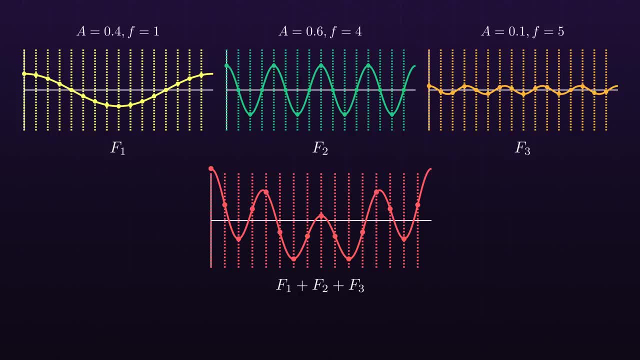 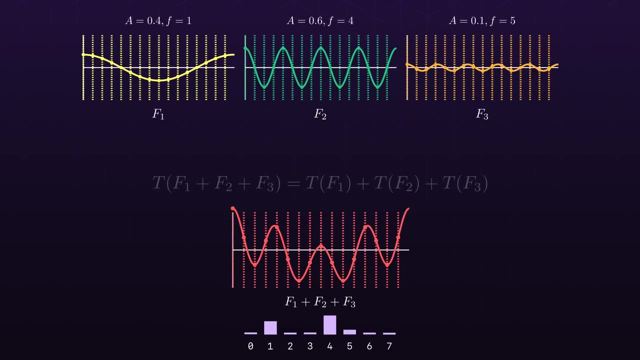 a signal of zero frequency and our transform properly extracts all the frequency components. We want our ideal Fourier transform to extract exactly these frequencies. When we pass the sample point from this signal into our test transform, we do indeed get those frequencies. The fundamental reason this works is that our transform is just a matrix multiplication. 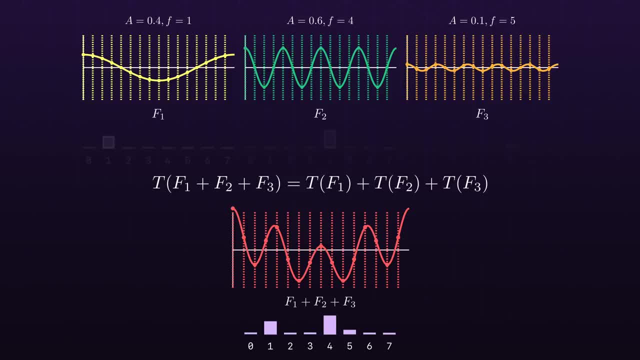 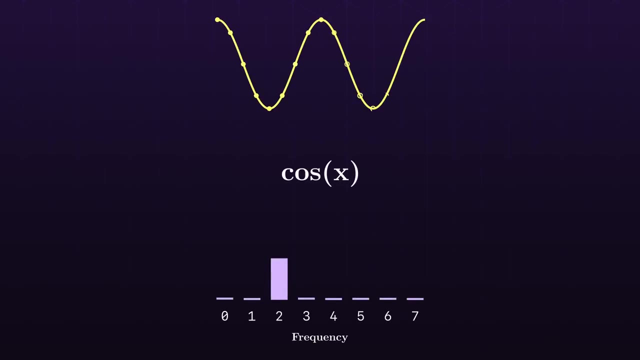 so it's linear. What that means is the output of this transform on this aggregate signal is exactly the same as if we performed the transform on the individual signal separately and then summed the outputs together. So far we've focused on cosine waves. Let's now see what happens when we use sine waves. 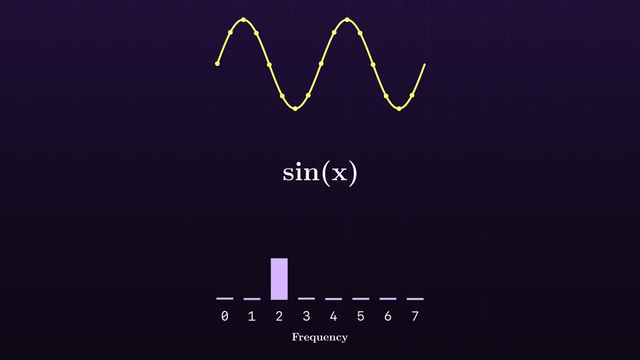 What we expect is, if we pass in a sine wave of some frequency, we should ideally get that same frequency displayed in our frequency spectrum. So let's try it. What we get is a bit surprising. It seems like all the frequency components are zero. And if we do some further digging, 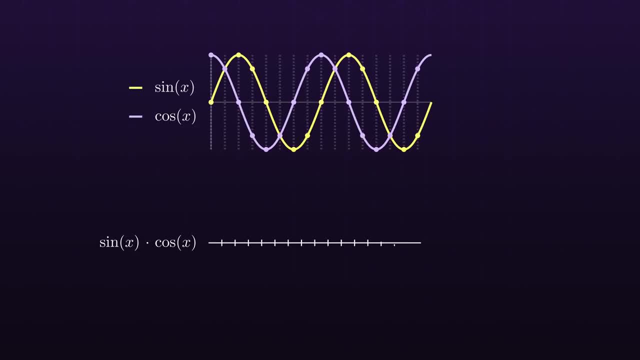 it turns out that if we take the dot product between this cosine wave analysis frequency and the matching sine wave frequency, the dot product is indeed zero. Interestingly enough, this is true for any frequency. Sine waves and cosine waves of matching frequencies are orthogonal to each other. Our test transform: 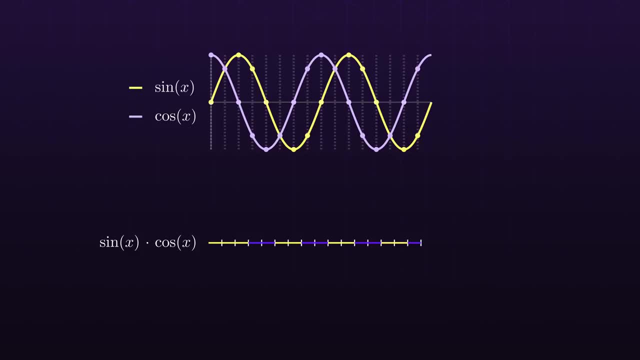 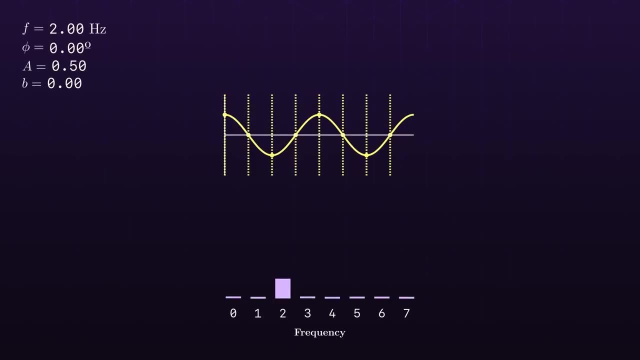 as currently constructed, will be unable to extract frequency information from sine waves. To understand what's going on, we have to go back to our test cases. We tested changing amplitudes, we tested changing frequencies and we also tested shifting the signals up and down. 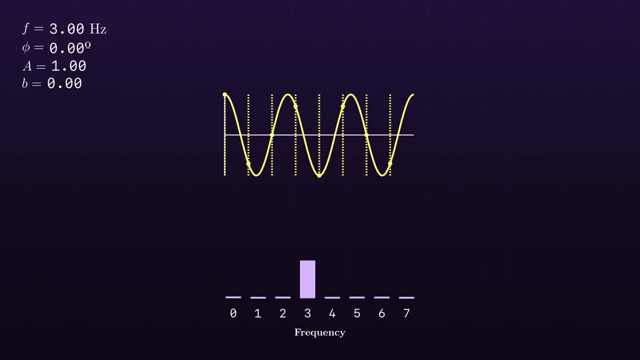 But one other component of signals that we can change is the phase. Remember: what we expect to happen when we change the phase is that our frequency component strength should stay the same. After all, it's the same frequency still present in the original signal, just shifted across time. But what happens with our test transform is unfortunately 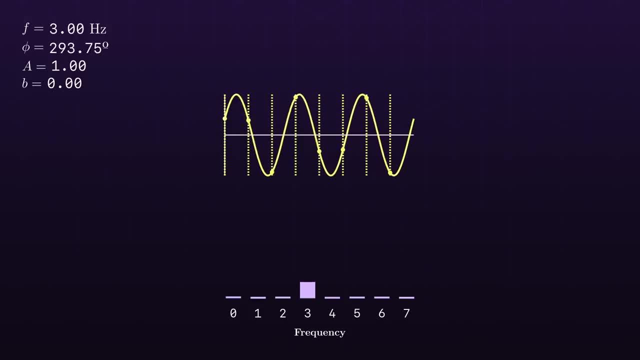 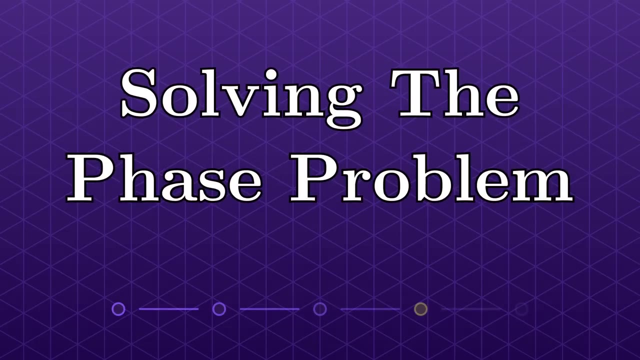 the frequency strength is impacted by the phase. The sine wave example is just a specific case, when the phase is offset by 90 degrees. So fundamentally, this is where our fake Fourier transform breaks. Let's now see how we can fix it, While in the case where we originally had a sine wave- one kind of hacky way to fix this. 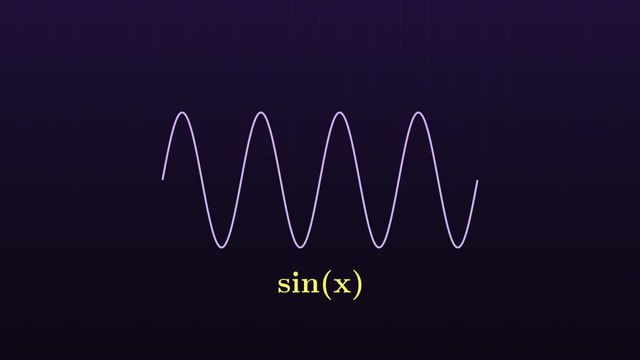 problem is to use analysis frequencies that correspond to sine waves instead of cosine waves. Now, with this sine wave version of the transform, every frequency sine wave properly gets a frequency contribution after going through our test transform. But, as you may expect, this breaks our original cosine wave comparisons. 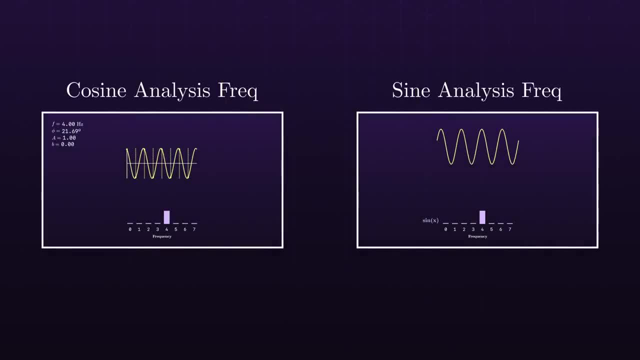 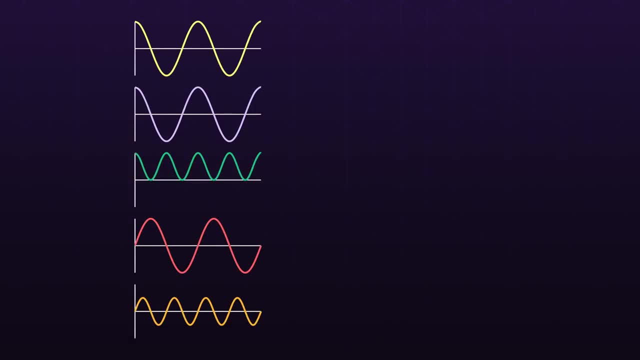 where we now end up with the same problem. So there seems to be some kind of balance that needs to be struck here. but how exactly can we do it? Well, let's play around with these separate cosine and sine wave analysis frequencies and see what. 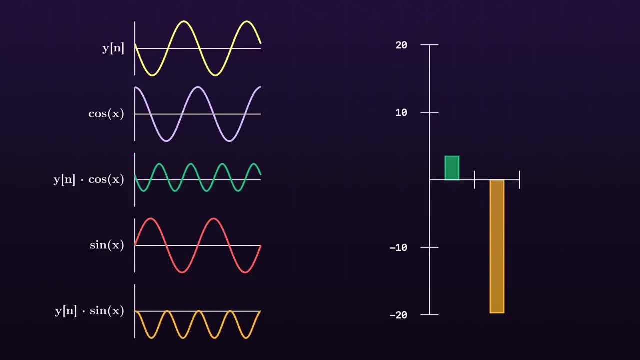 happens Given a signal, let's modify the phase of the signal and capture values from both the cosine and sine versions of our fake transforms. What's going on here is we are capturing the dot product of the matching analysis frequency for our original signal for both versions of these transforms. 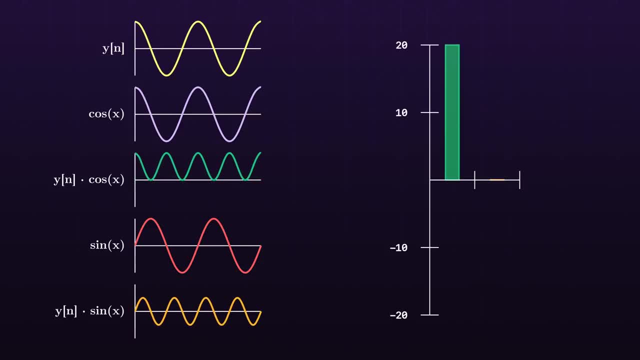 As you can see, when the underlying wave is a cosine wave, the cosine component dominates. When the phase is altered to a sine wave, the sine component takes over. One thing that's kind of interesting here is these values are never simultaneously zero, and there's also a fun sort of dance going on between. 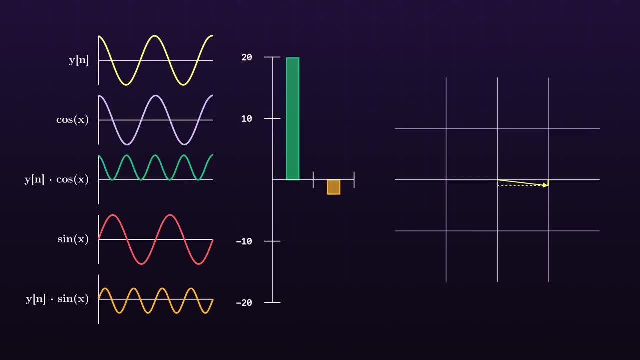 them. One idea that seems interesting is to see what happens when we plot these values on a 2D coordinate plane, And what's pretty interesting is we see that these coordinates trace a circle as we change the phase of the original signal. How cool is that. 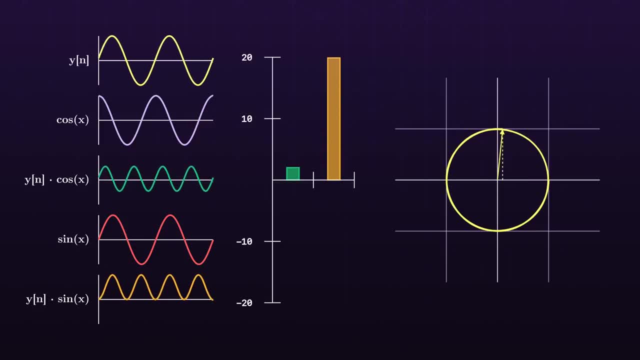 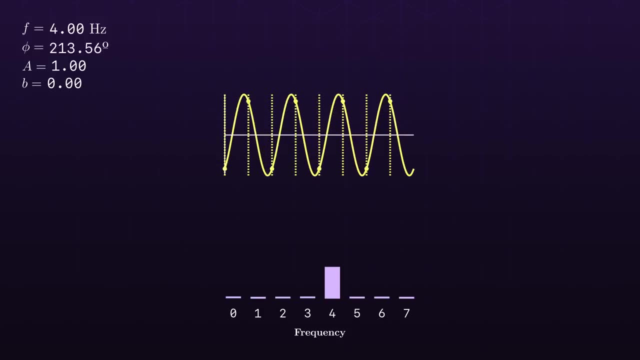 But the question remains: how do we put this together in a way that solves our phase problem? As a reminder, the original issue we're trying to solve here is, as we were changing the phase of the signal, we were getting different frequency contributions from the test transform. 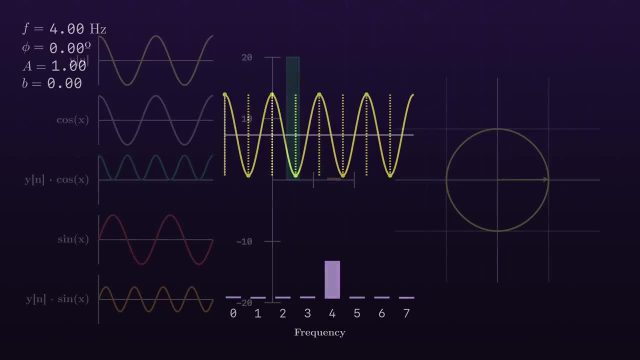 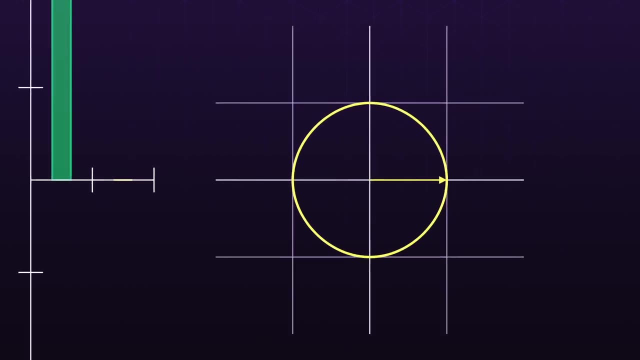 What we want ideally is a way for our frequency contribution to stay the same regardless of phase. Can we use a feature of these coordinates that trace a circle to give us a value that stays the same regardless of the phase? As some of you might have already guessed, it's the radius. 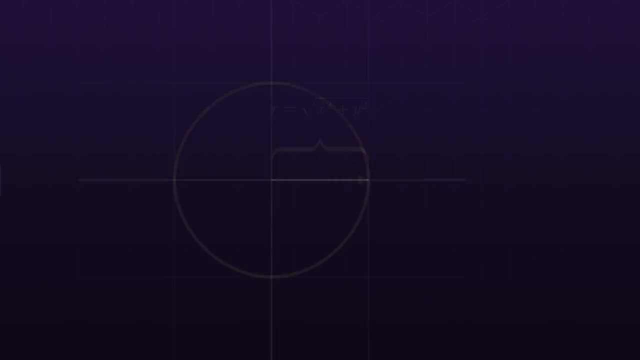 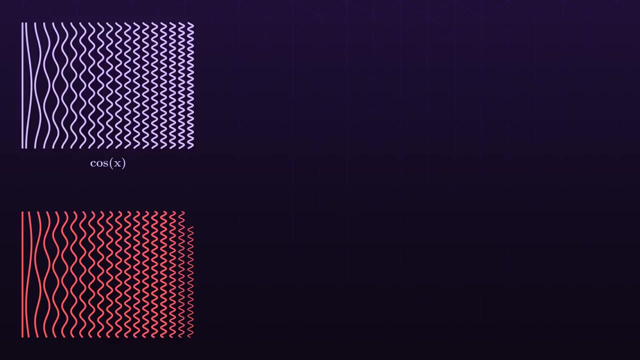 or, more concretely, the magnitude of these coordinates. So let's put this together into a new proposed solution. We originally had a matrix containing analysis frequencies of cosine waves. Now, what we'll add to the equation is a similar matrix, but for sine waves of different analysis. 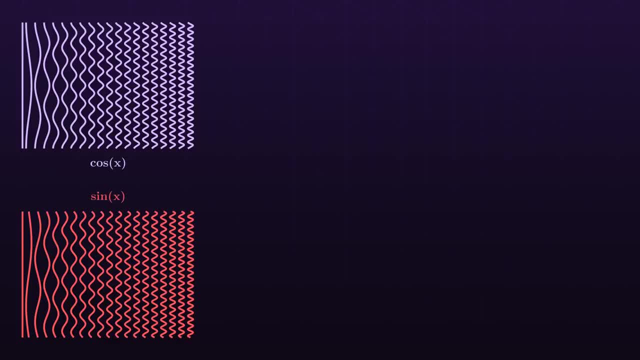 frequencies. The big idea now is that we can apply the cosine wave analysis frequency matrix to give us x coordinates and then apply the sine wave analysis frequency matrix to give us y coordinates. The final frequency domain representation will put these two coordinates together via the magnitude of these coordinates. 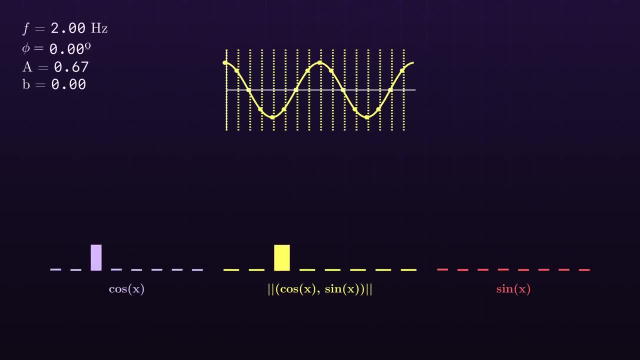 Here is the final combined version of this transform applied to our previous test cases. This combined version of sine and cosine analysis frequencies, by the way, is what most people refer to when they talk about frequency domain representations of the true discrete Fourier transform. But the DFT uses one more trick to simplify things: After all, generating these two matrices. 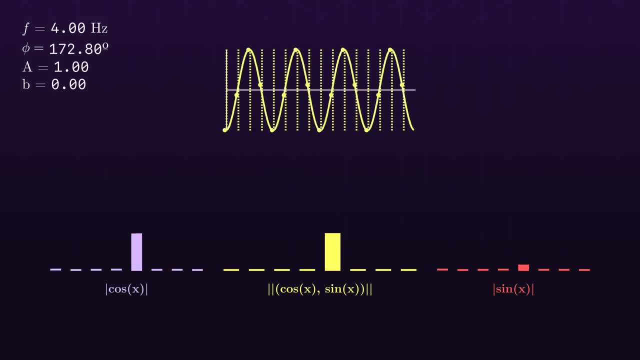 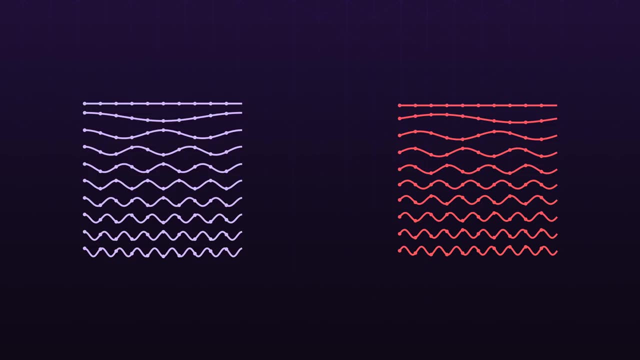 performing this transformation twice and then extracting the magnitude is a bit convoluted, a bit convoluted. The key insight is, instead of keeping track of two matrices that have sampled points from cosine and sine waves, we can jointly represent the two coordinates as sampled points from. 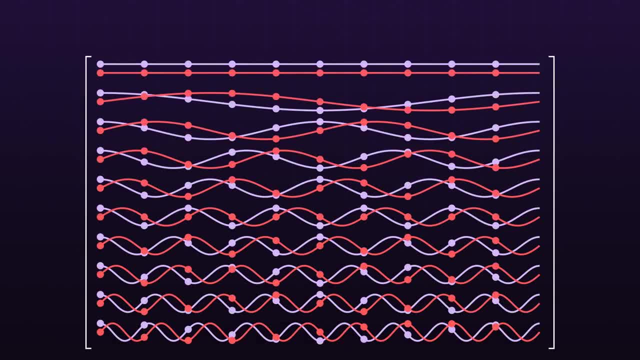 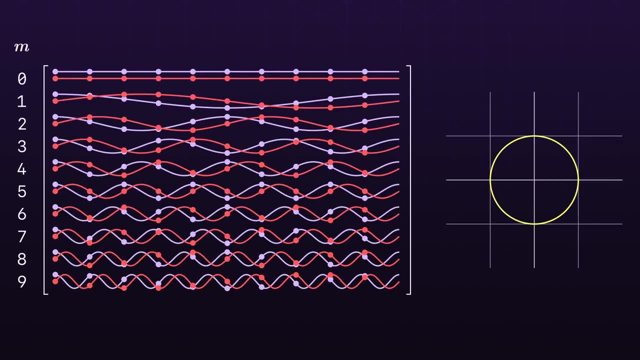 a unit circle into a single matrix. So let's see how this actually works for a signal with 10 sampled points. Breaking down an example is one of the best ways to see the underlying pattern For the analysis frequency 0, all the points are simply the same coordinate. 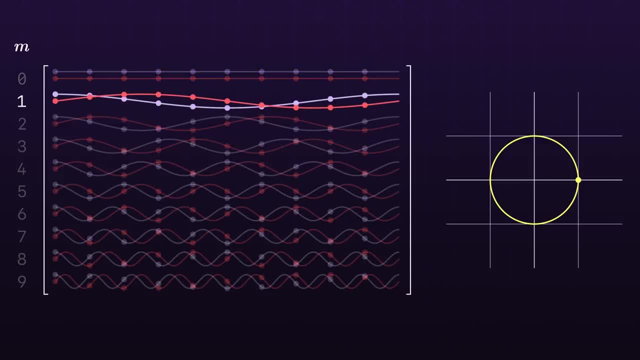 It's a zero frequency signal, so this is expected For the analysis, frequency 1,. things get more interesting If we plot the corresponding points from our cosine and sine samples. we get the following 10 points And, intuitively, what's going on here is we are taking a single cycle through the unit. 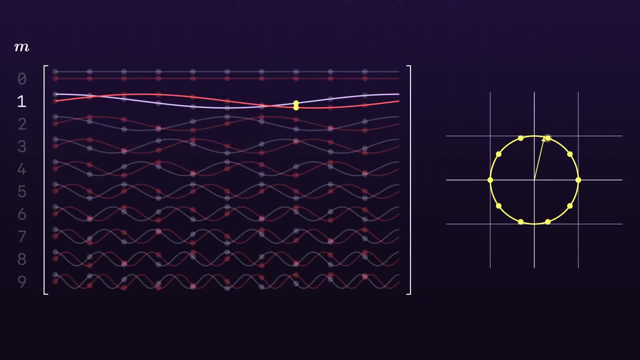 circle and uniformly sampling points until we get 10 points For the analysis. frequency 2, the points from the sine and cosine waves align as follows: And once again a nice way to interpret this is: we are regularly sampling points from the unit circle. but now the key difference. 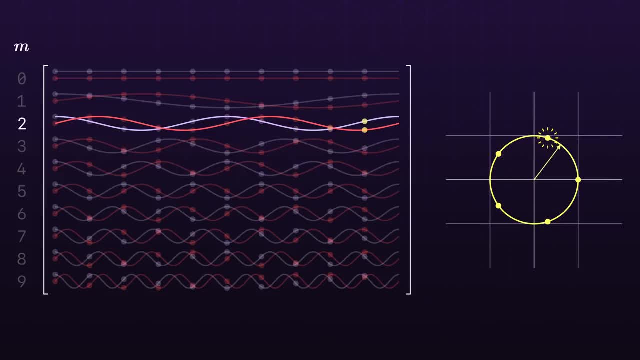 is. we do it over two cycles. Let's do analysis- frequency 3, to make sure the same pattern holds. We plot the sine and cosine points as before and what we again see is that they are uniformly sampled points from the unit circle with an underlying frequency of three cycles. 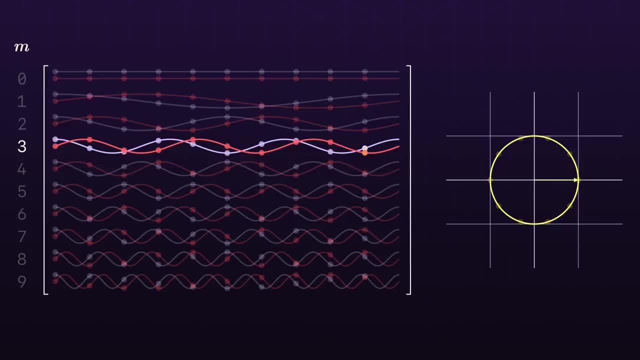 This pattern actually ends up continuing over all an analysis frequencies. The key interpretation here is that each analysis frequency samples points from the unit circle in a uniform manner, with an angular frequency that matches the analysis frequency. The final part of the simplification to the true DFT is when we discuss points on a unit. 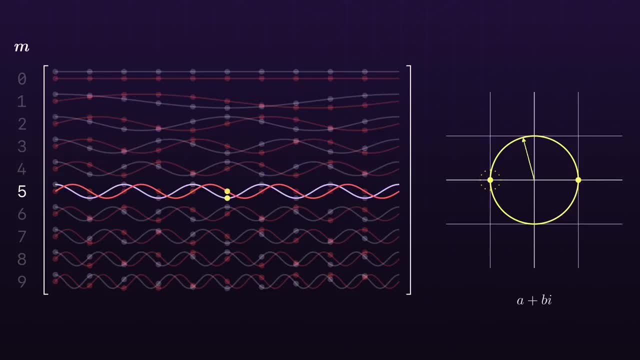 circle. it's quite convenient to represent the coordinates as complex numbers. The real components of these complex numbers correspond to points on the original cosine wave. The primary components are mapped to points on the original sine wave. In practice, these points are compactly represented as complex exponentials via Euler's formula. 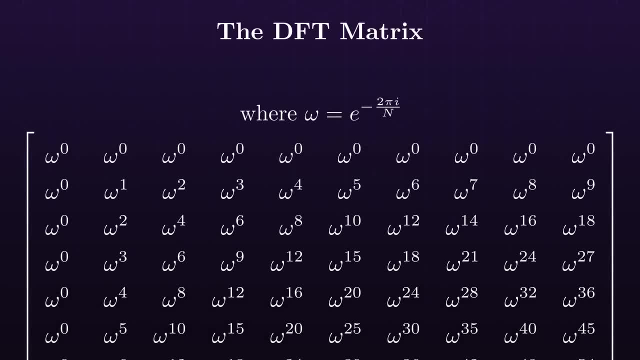 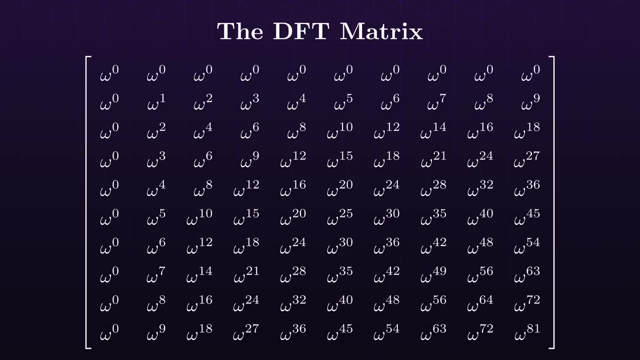 The final DFT matrix is composed of complex exponentials where every row corresponds to sample points from the unit circle at distinct integer analysis frequencies. Thanks for watching. See you next time, Bye. 1 matrix is by defining it as complex exponentials regularly sampled from the unit circle. 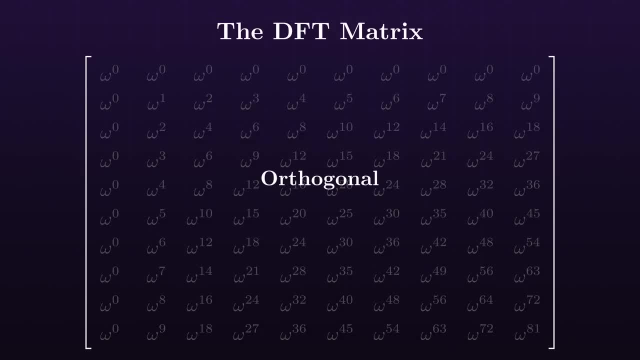 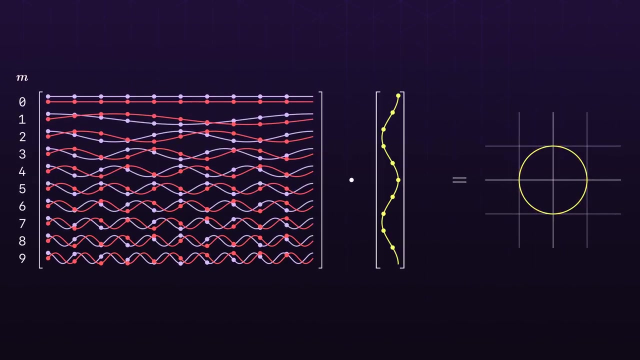 it's actually an orthogonal matrix. This matrix, as a result, ends up satisfying all the requirements we were looking for when we started this journey. So taking a step back, the DFT is fundamentally just a matrix vector product of a time domain signal with the DFT matrix. When you multiply this matrix with your time domain signal, 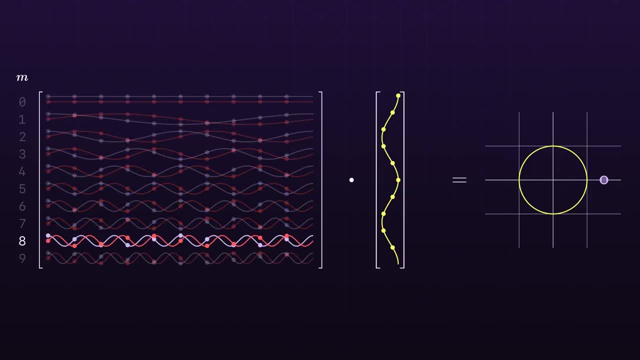 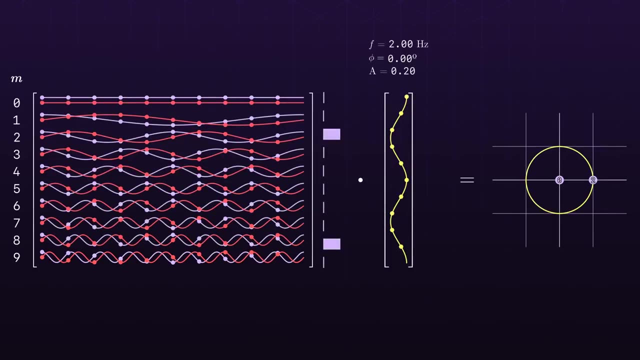 you get a sequence of complex numbers. The magnitude of each of these complex numbers tells you the contribution of that respective analysis frequency throughout the original signal. The angle of the complex coordinate is a measure of the phase of the signal. The best way to see this is with our previously failing test case. 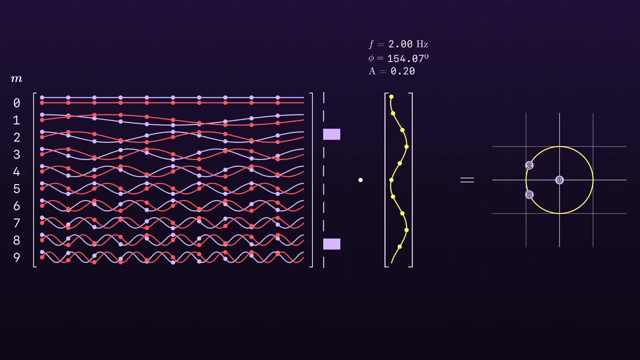 When we perform the DFT, transform and plot the magnitude of the frequency components, we can see that the magnitudes of the peaks do not change as the phase of the signal changes. But what's really cool is the angle of these corresponding peaks, when plotted on a complex plane, correspond exactly to the phase of the signal at that frequency. 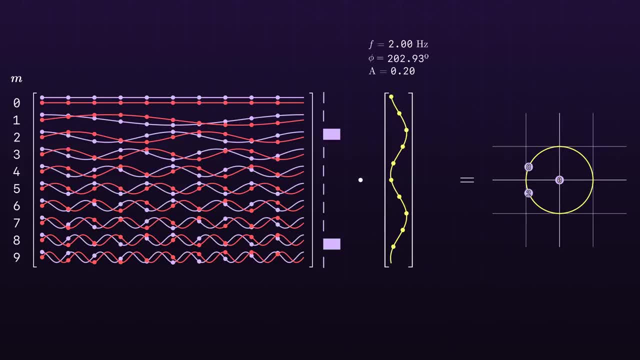 This is how the DFT uniquely captures frequency contributions and phase in a signal. Earlier we talked briefly about how there are 2 peaks in the full spectrum of a cosine wave when we use our fake transforms. The true DFT also has this property for real. 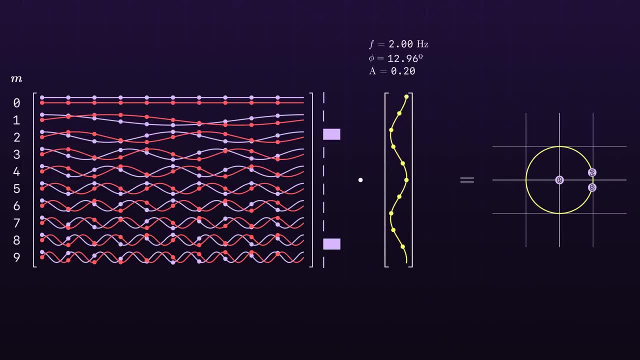 valued cosine waves. But now the interpretation is a bit different. The DFT decomposes a signal into a set of complex exponentials. The first peak corresponds to a complex exponential that has an underlying frequency matching the original cosine-weight frequency, while the second peak corresponds to a complex exponential. 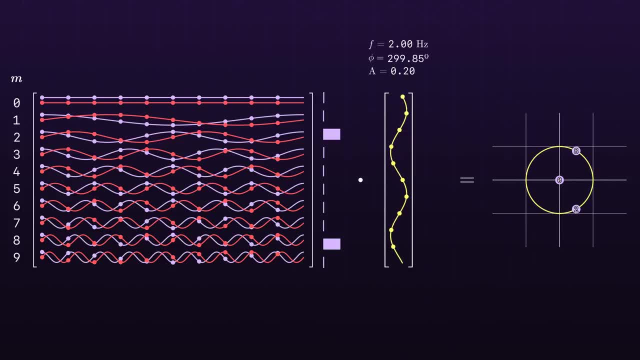 that has an underlying frequency that is moving in the opposite direction and perfectly cancels out the imaginary component of the first complex exponential. And this will always be the case for all real-value signals. This symmetry is required to cancel out the imaginary components and get a real signal. 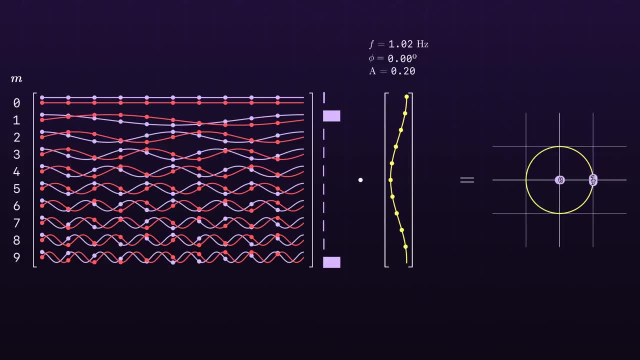 A final example that's also helpful to gain intuition on what's going on in the DFT is notice how, as we change frequencies of our test signal, when the test signal matches one of our analysis frequencies in our DFT matrix, the values from the respective analysis frequencies shoot out, while all the other frequencies. 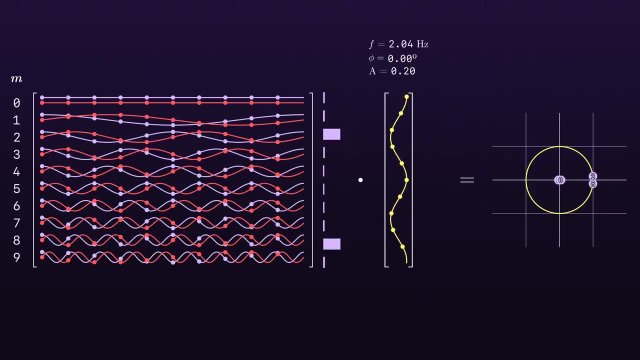 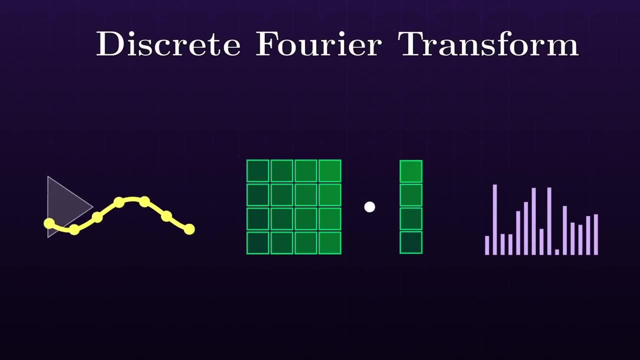 are centered around zero. This is another way to visualize how our earlier measure of similarity materializes now in a complex plane. From an implementation perspective, the DFT is fundamentally just a matrix-vector product and the inverse DFT- to get the original signal back- is also a matrix product, with the inverse.